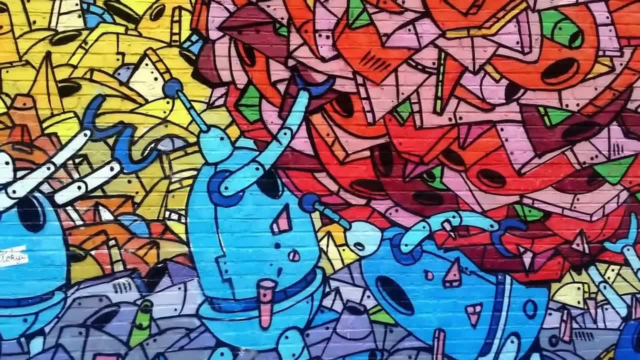 Quantum mechanics is the idea of the absurd. Strange explanations like wave-particle duality, the uncertainty principle and the collapse of the wave function. 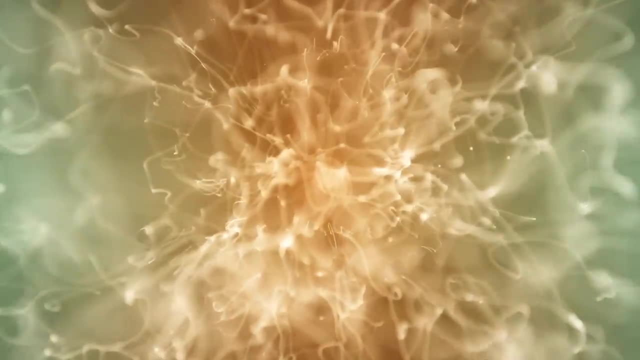 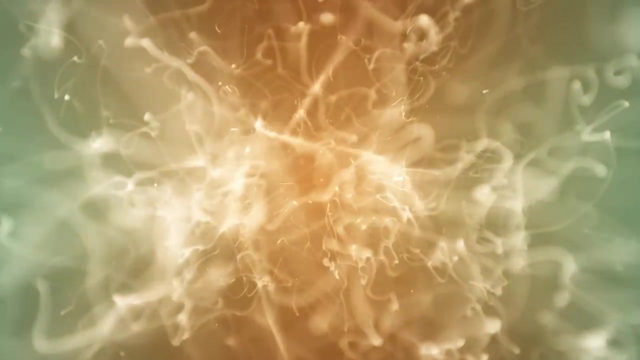 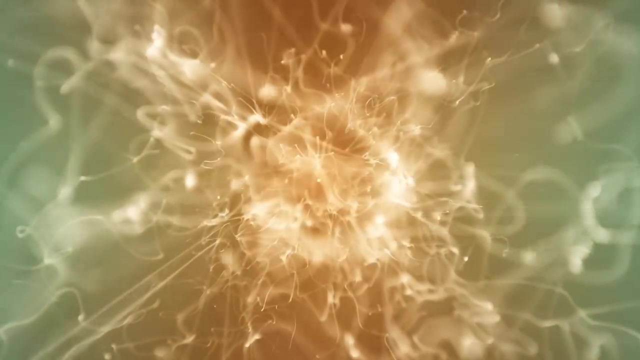 Things become even stranger when we consider the quantization of the electromagnetic field, including the polarization of the quantum vacuum, electrons and photons interacting with their own electromagnetic fields, particles travelling back in time, the emission and reception of virtual photons or the continuous creation and destruction of electron-positron 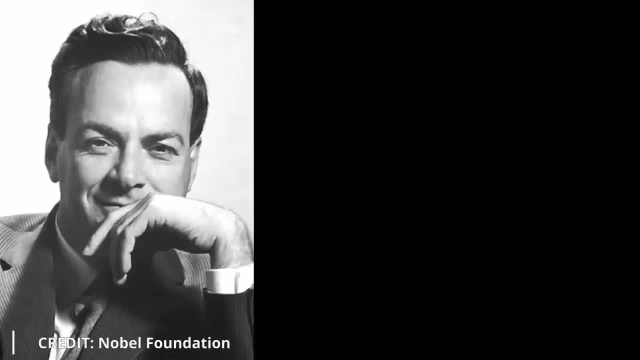 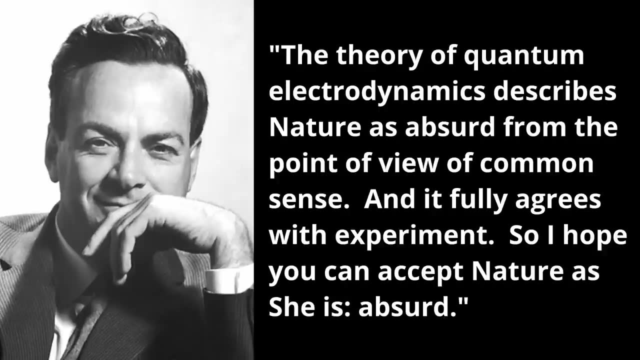 pairs in a quantum vacuum. Feynman summed it up as follows. The theory of quantum electrodynamics describes nature as absurd from the point of view of common sense, and it fully agrees with experiment, so I hope you can accept nature as she is absurd. 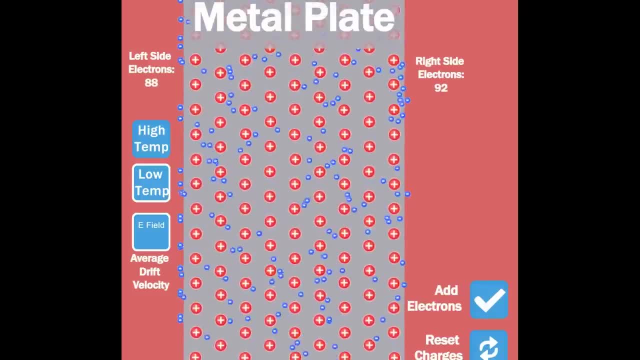 Electrodynamics is the branch of physics that deals with the effects arising from the interaction of the quantum vacuum. 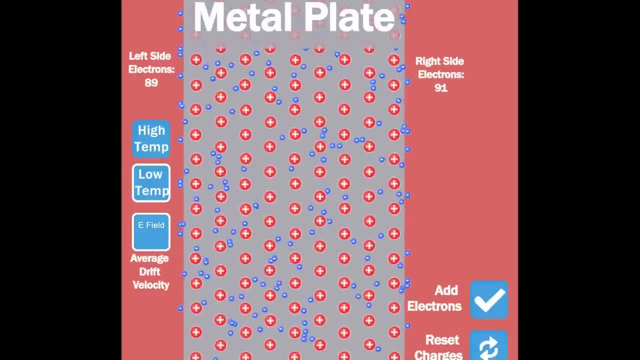 Electrodynamics is the branch of physics that deals with the action of electric charges and currents using an extension of the classical Newtonian model. 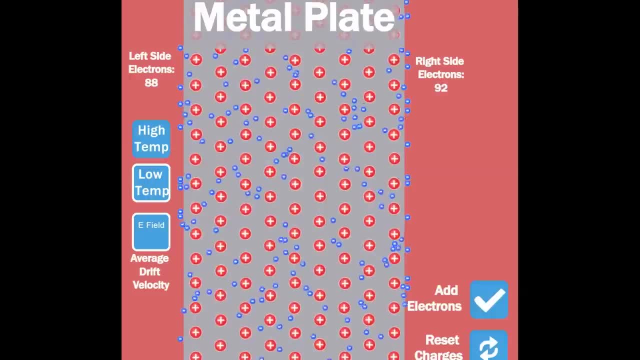 It provides a description of electromagnetic phenomena whenever the relevant length scales and field strength are large enough that the quantum mechanical effects are negligible. 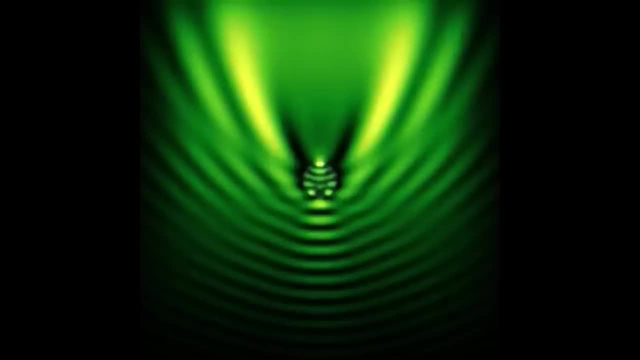 For small distances and low field strength, such interactions are better described by quantum electrodynamics. In essence, it describes how light and matter interact. 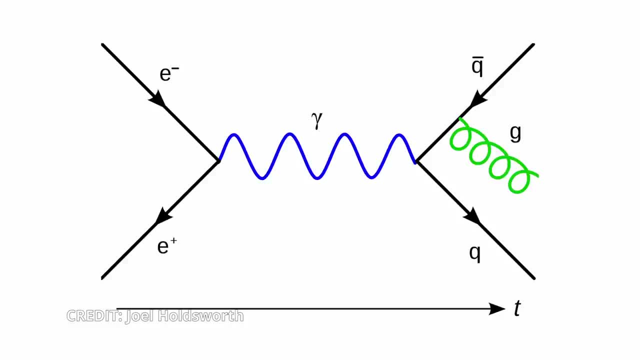 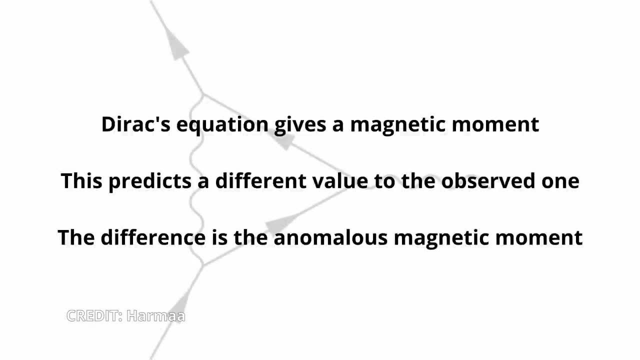 Quantum electrodynamics is considered the most accurate theory in the history of science. The precision is all based on a single experimental value, the anomalous magnetic moment of the electron called the g-factor. 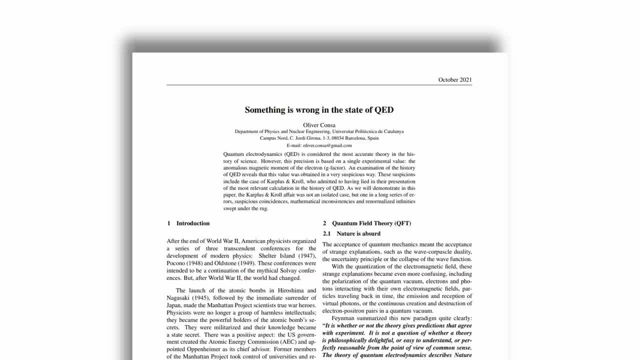 In this episode, I want to examine a paper by Oliver Konzer, who examines the very suspicious coincidences, errors, mathematical inconsistencies, and renormalization of infinities which have been swept under the rug. 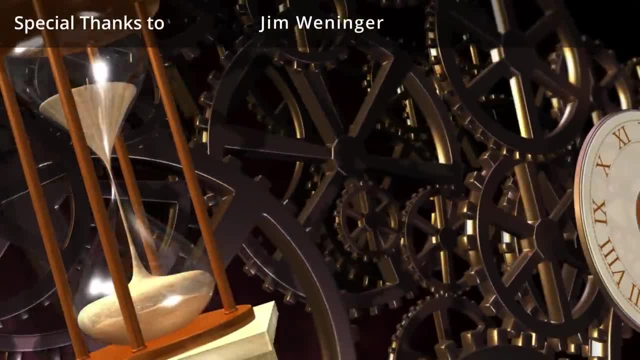 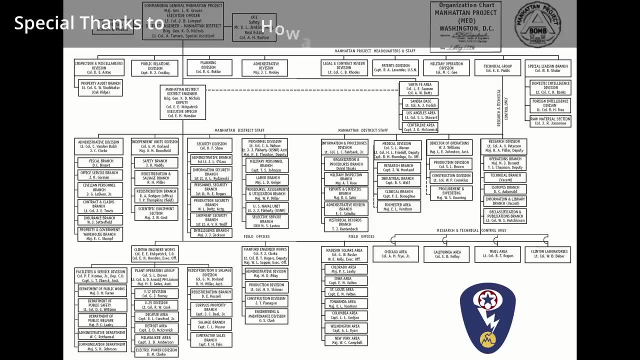 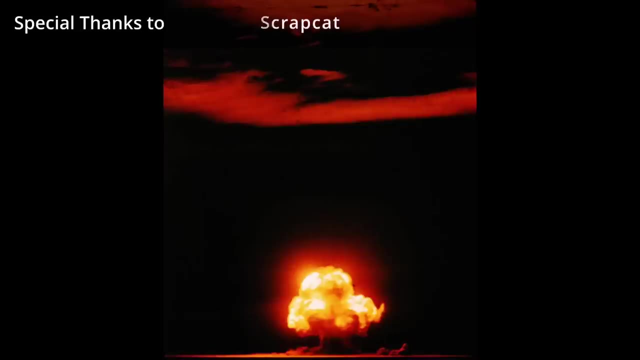 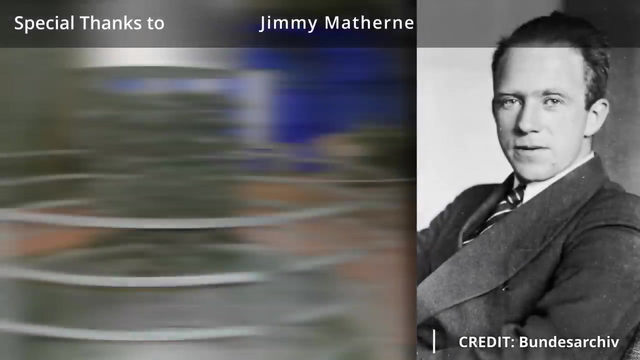 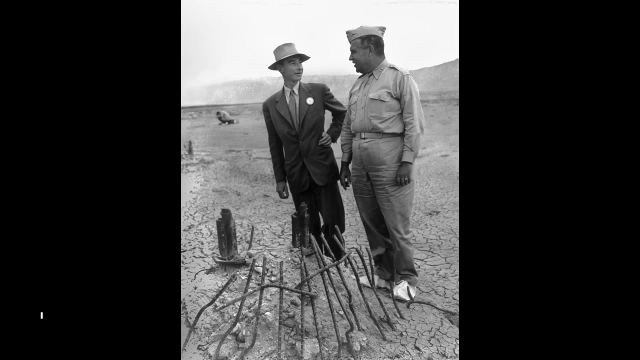 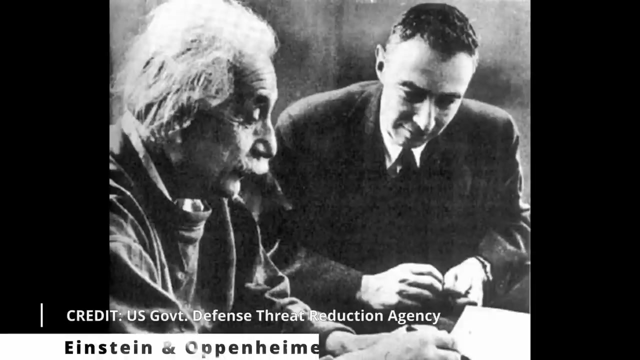 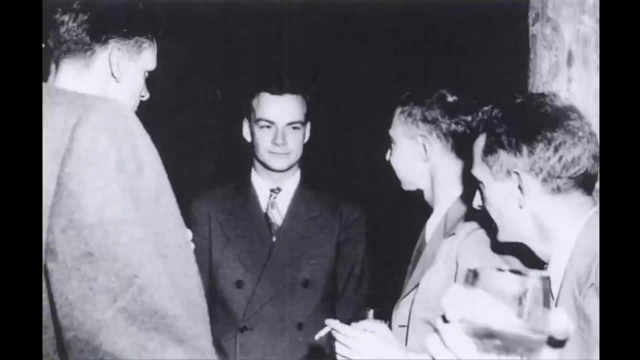 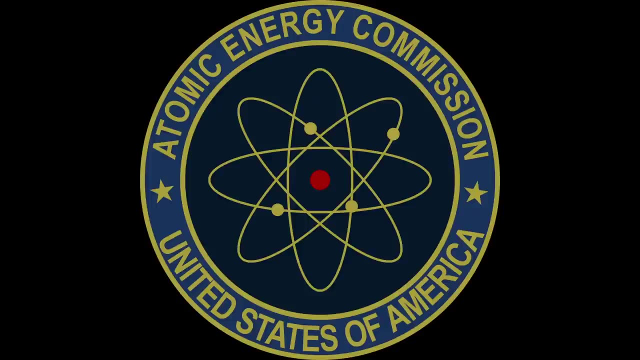 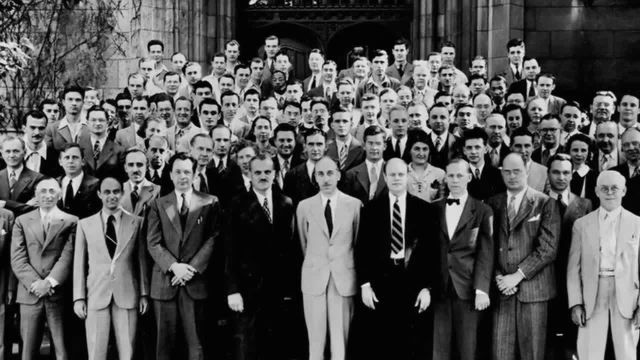 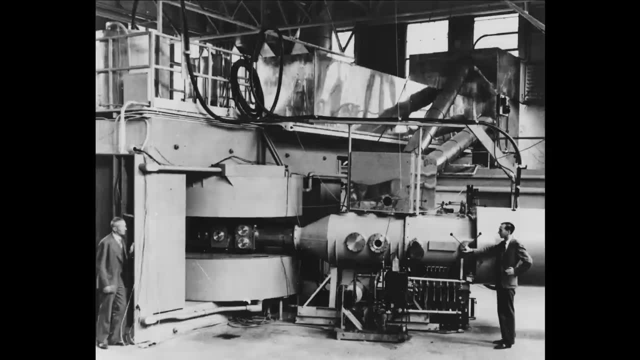 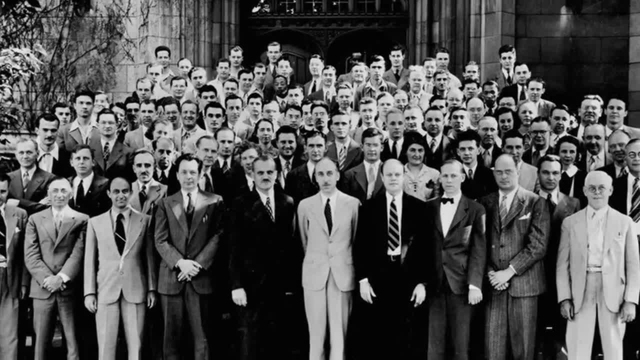 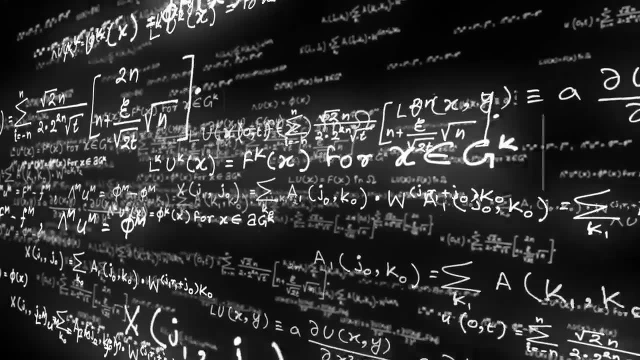 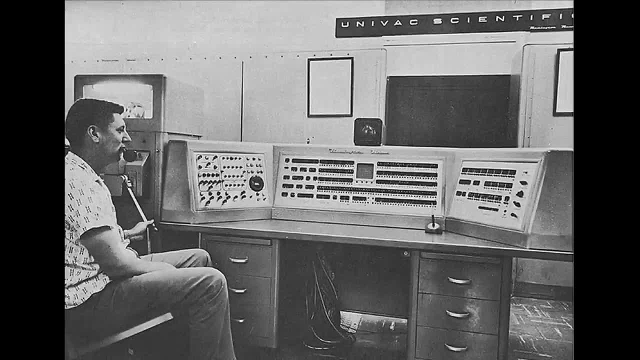 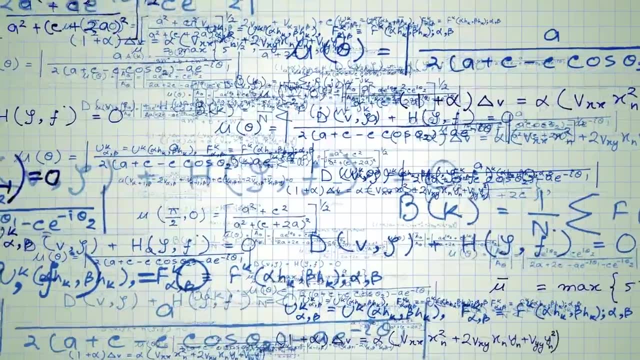 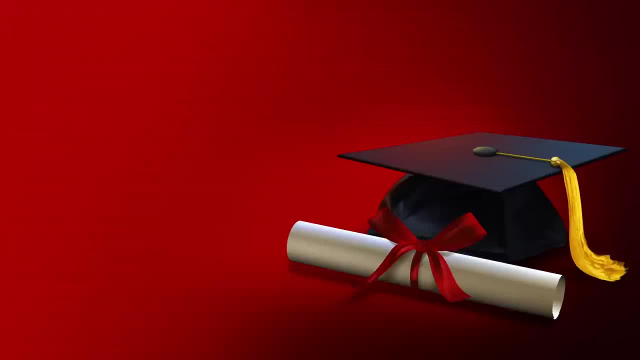 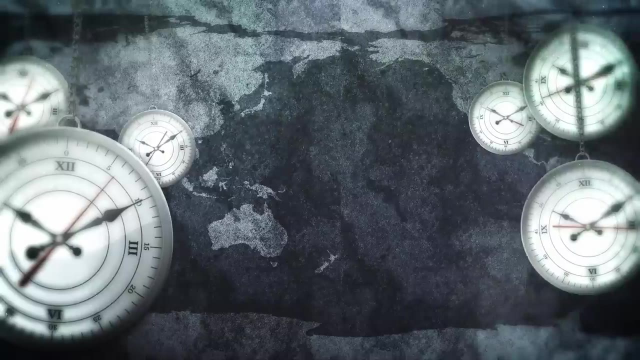 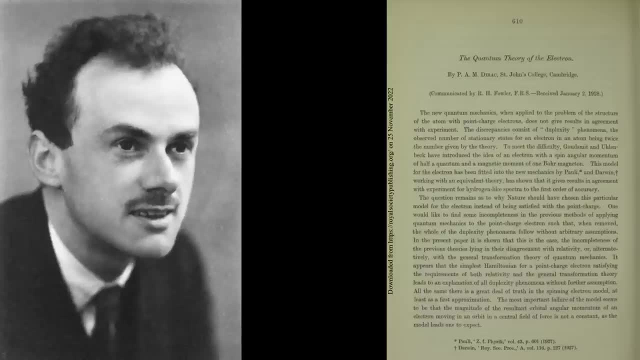 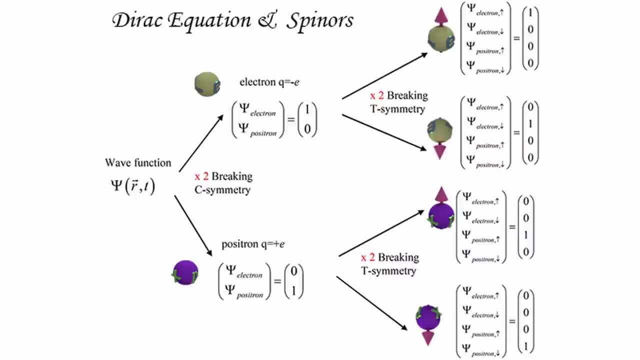 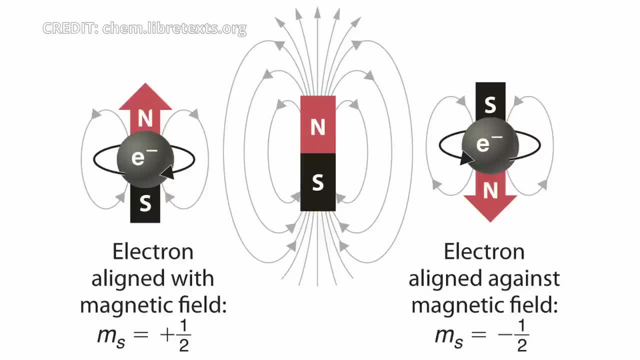 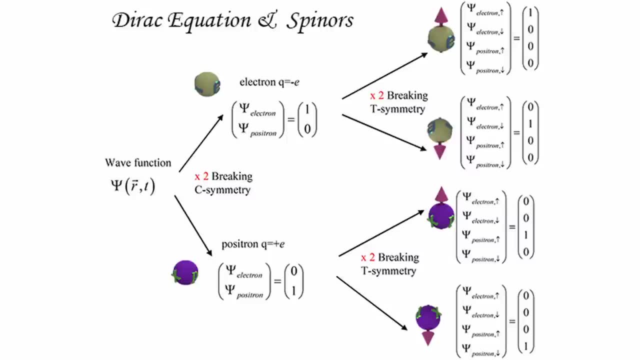 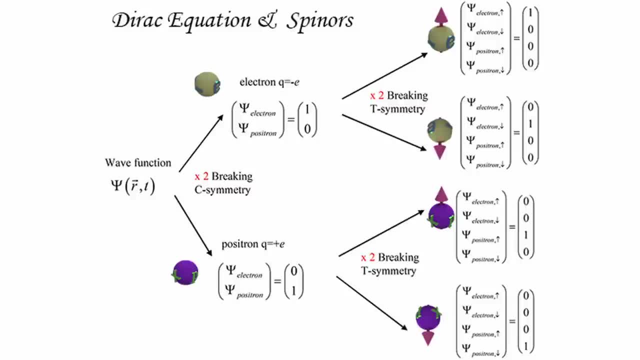 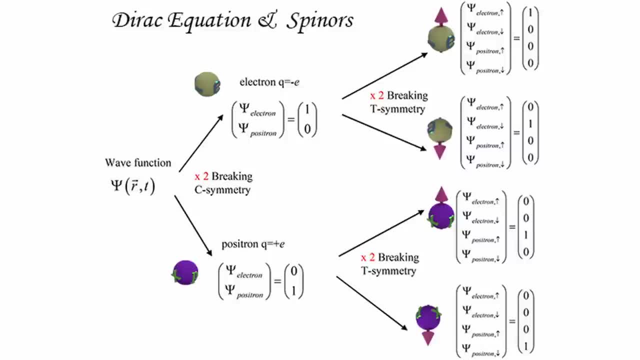 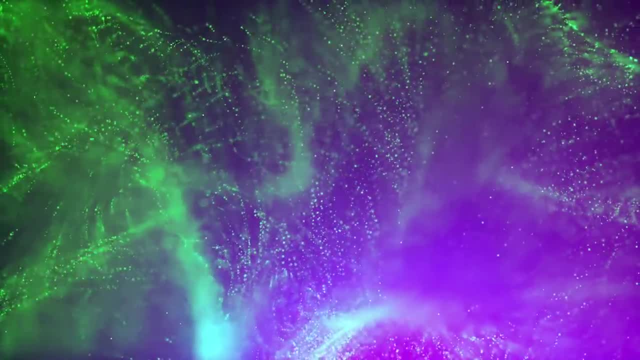 there was a counterpart to the electron, the antielectron or positron. Based on the success of Dirac's equation, quantum mechanic theorists attempted to quantify the 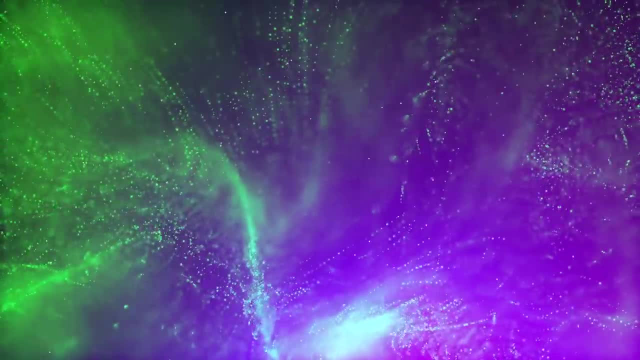 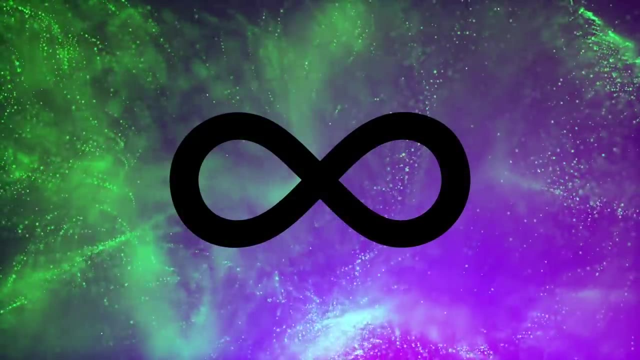 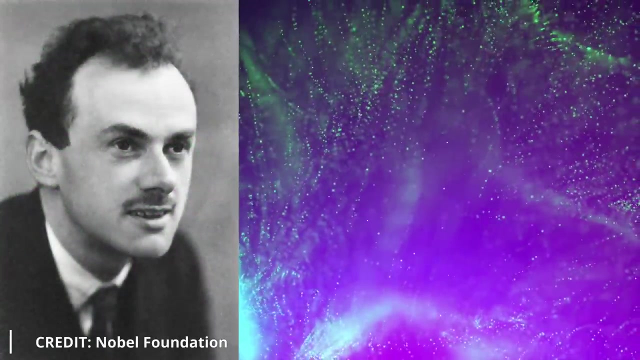 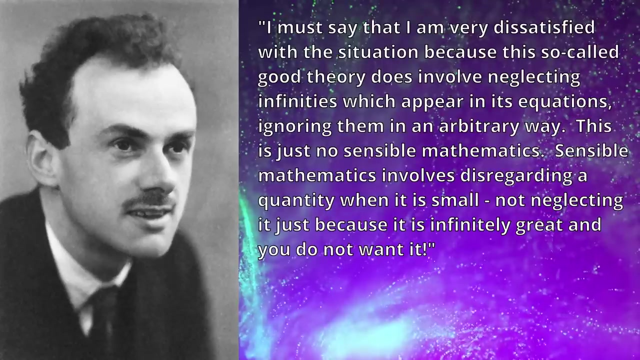 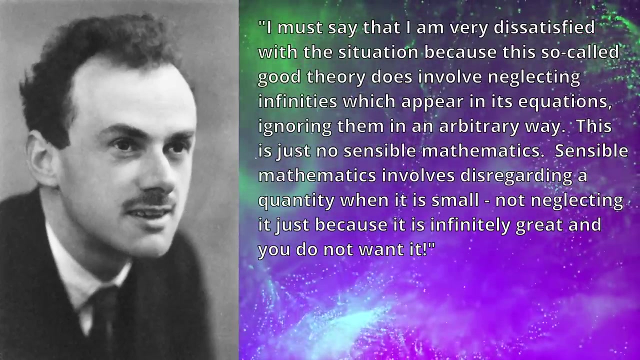 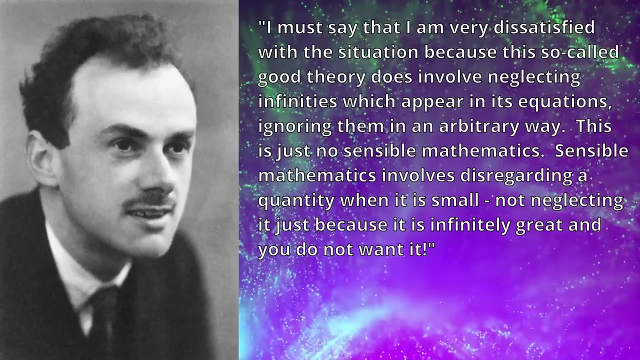 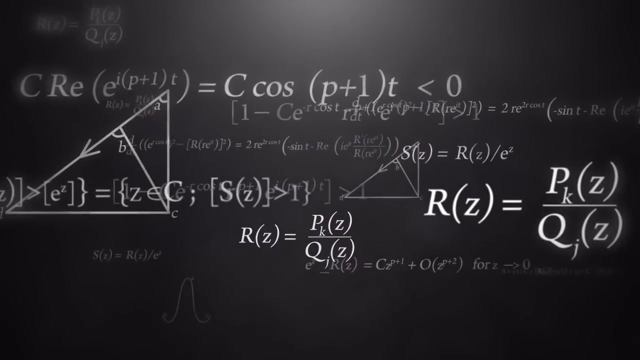 electromagnetic field by creating the quantum field theory. All attempts at this seemed to fail as calculations under this theory resulted in an infinite number. Their solution to this problem was to simply ignore these infinities. Dirac was horrified by this saying, I must say that I am very dissatisfied with the situation because this so-called good theory does involve neglecting infinities which appear in its equations, ignoring them in an arbitrary way. This is just no sensible mathematics. Sensible mathematics involves disregarding a quantity when it is small, not neglecting it just because it is infinitely great and you do not want it. The technique of ignoring infinities is called renormalization. 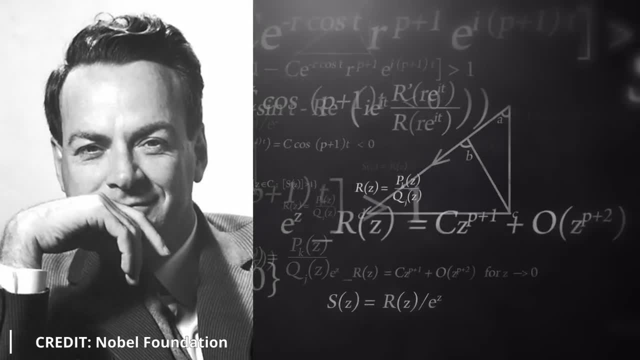 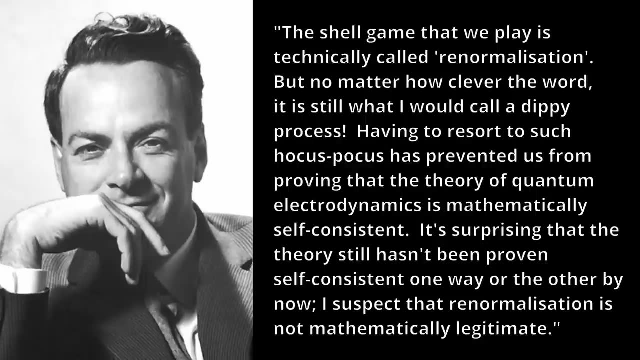 Even Feynman recognized that it is not a mathematically legitimate technique, stating, It's surprising that the theory still hasn't been proven self-consistent one way or the other by now. 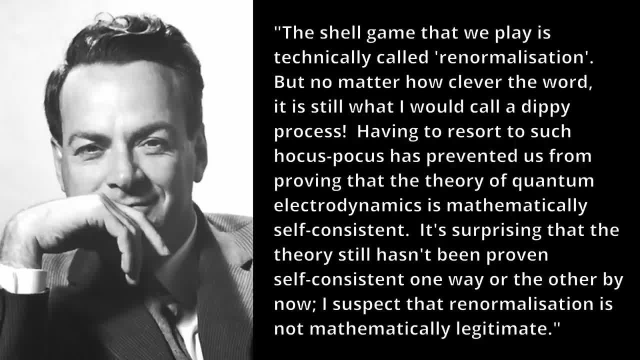 I suspect, that renormalization is not mathematically legitimate. 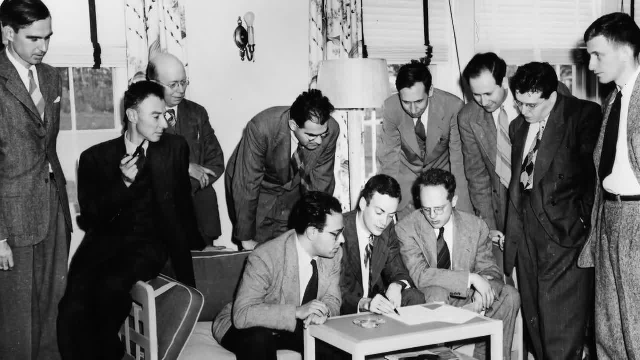 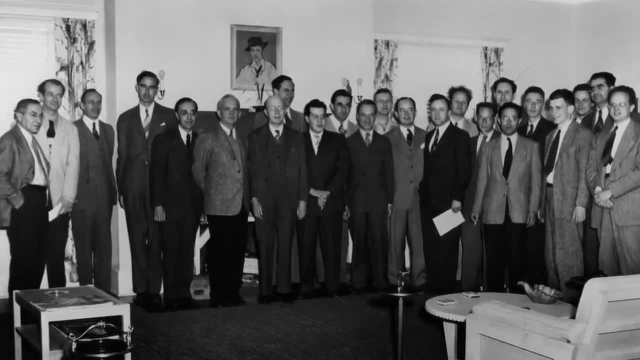 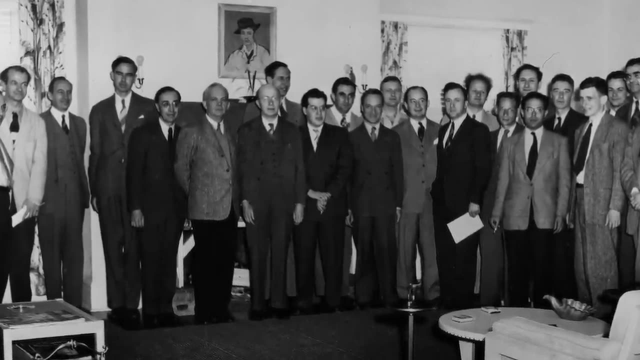 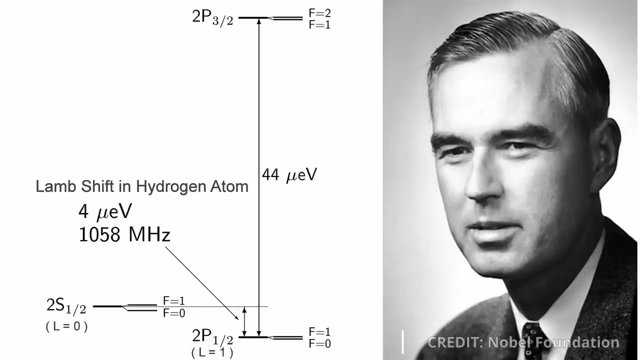 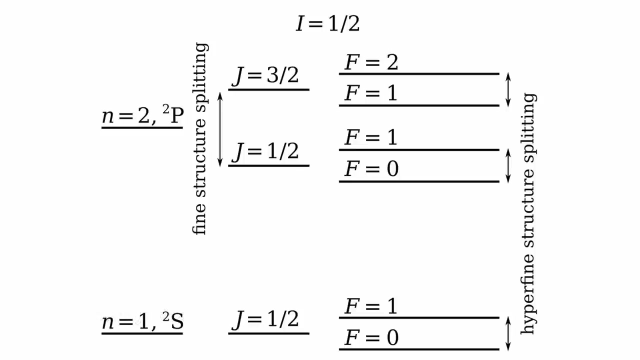 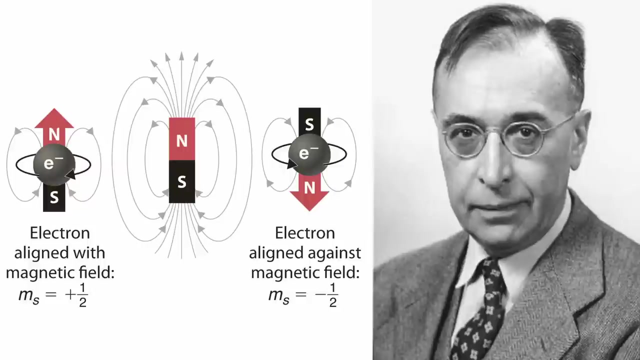 In June of 1947, the first International Physics Conference after World War II was held at Shelter Island. It brought together 24 physicists from the Manhattan Project. The participants were received as celebrities and it made a significant impact in the press. Two important experimental measures were presented. In the first, Lamb presented an experiment that showed the 2s-half energy levels of an electron are not identical. Instead, they differed by 1000 MHz. The other experiment showed a 0.1% anomaly in the hyperfine structure of hydrogen. Later, Bright would interpret this anomaly as the anomalous magnetic moment of an electron, called the g factor. 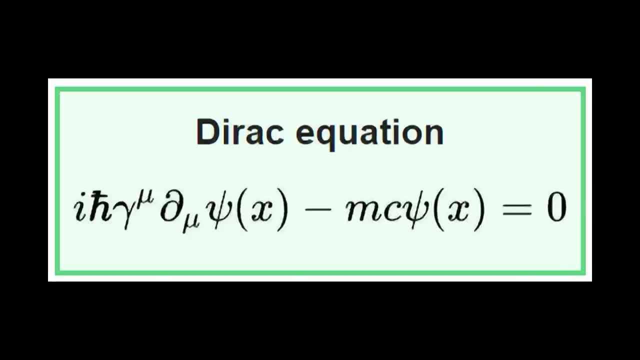 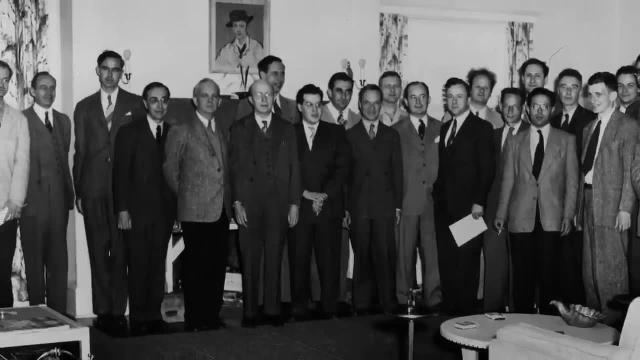 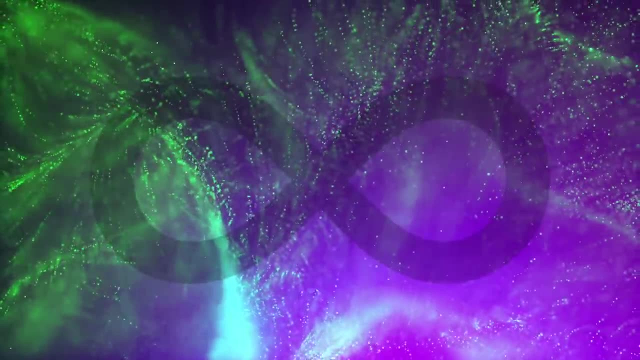 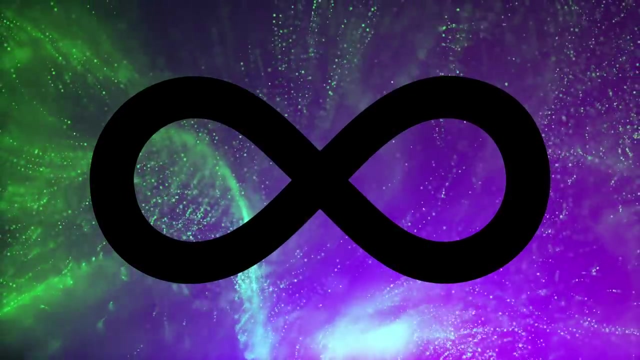 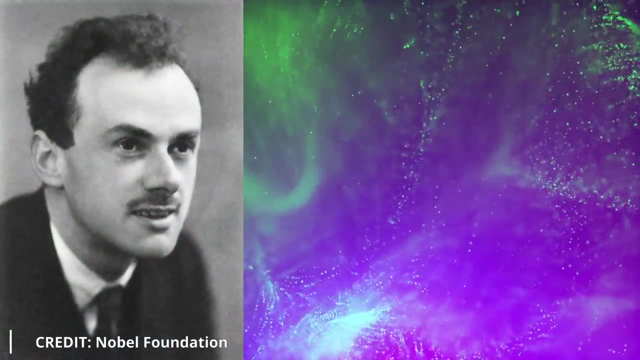 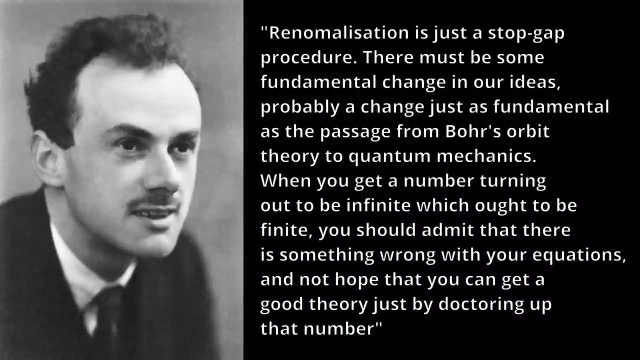 The problem was that both of these measurements contradicted the Dirac equation. To the meeting participants assumed Dirac's theory of the electron must be slow. They were not able to show the must be incomplete and proposed that these effects were due to the quantization of the electromagnetic field. They also assumed that the discrepancy could be calculated using quantum field theory and that the infinities of that theory could be corrected using renormalization techniques. This is the origin of quantum electrodynamics. Sadly, Dirac was not at the conference and took a very dim view saying renormalization is just a stopgap procedure. There must be some fundamental change in our ideas, probably a change just as fundamental as the passage from Bohr's orbit theory to quantum mechanics. When you get a number turning out to be infinite, which ought to be finite, you should admit that there is something wrong with your equations and not hope that you can get a good theory just by doctoring up that number. 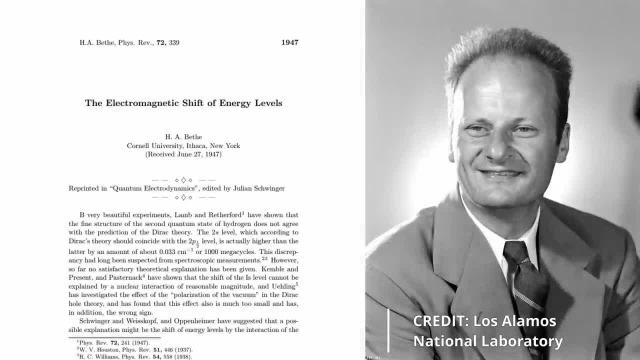 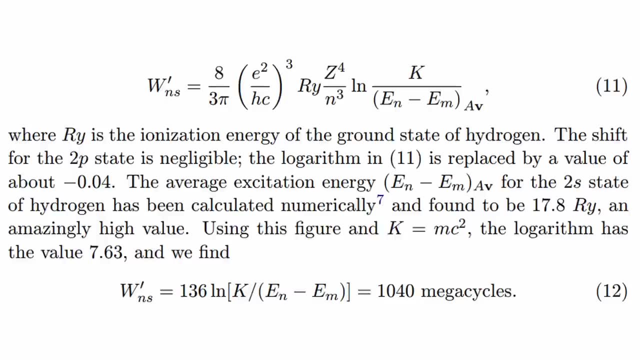 A little while after the conference, Beter published a paper outlining an equation for the Lamb shift. And here is the equation. What is important is that the value of k on the right hand side diverges to infinity. So Beter decided to apply renormalization by substituting the infinite values for the finite value of the electron's energy, so k equals mc squared. The problem is that there is no physical justification for making this change. The only reason to use it is that 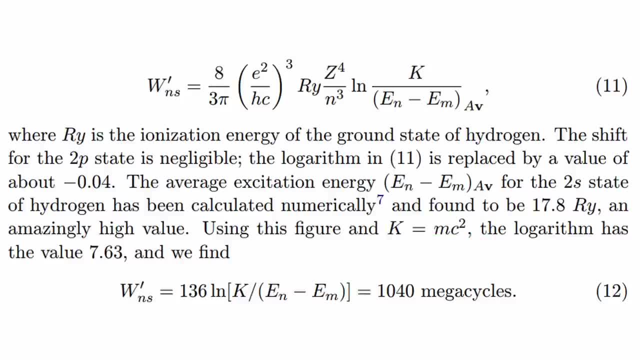 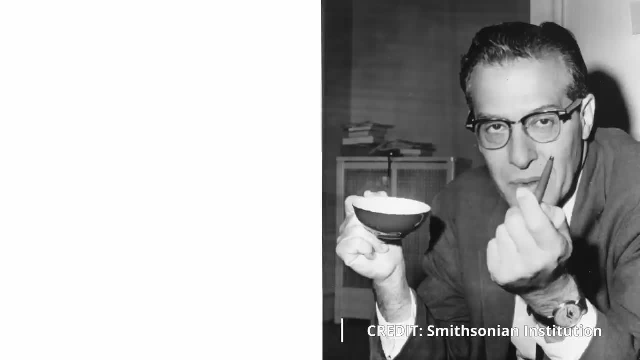 the final result do yield a value that was close to the experimental value. A few months after Beter's paper, Schwinger attempted to calculate the g factor for the electron. Here is his equation for g. 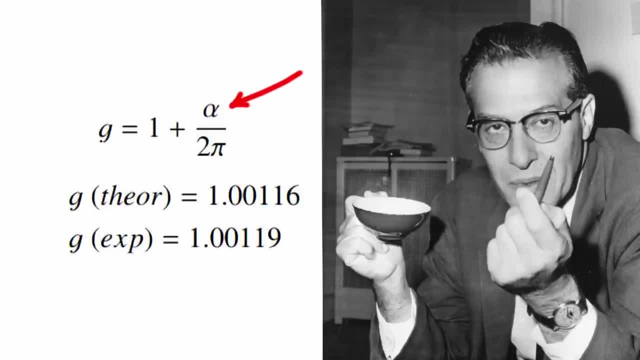 Here alpha is what is known as the fine structure constant. It is a fundamental physical constant. It effectively determines the size of the splitting of the fine structure of the hydrogen spectral lines. It was considered to be important under Dirac's linear relativistic wave equation, which gave the exact fine structure formula. 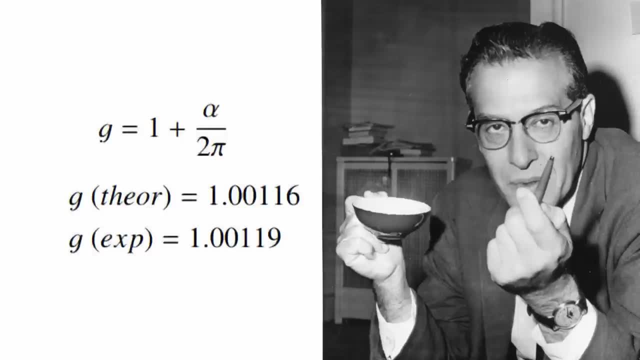 Schwinger's experiment seems to be very close to the experimental value, which had previously been published. He never explained how he derived his equation, and stated that he would publish a paper outlining the details of his theory soon. Schwinger had assumed that the g factor should be directly related to the fine structure constant, which has an approximate value of 0.7%. Dividing this value by 6 or 2 pi, provides an approximate value of 0.1%, which is the value that had been obtained experimentally. I hope you enjoyed this video. If you did, please leave a like and subscribe, and I will see you in the next video. 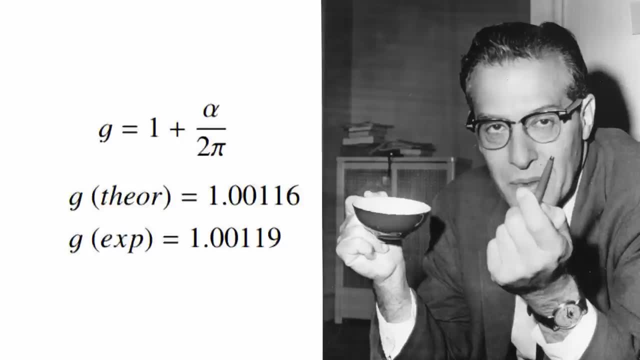 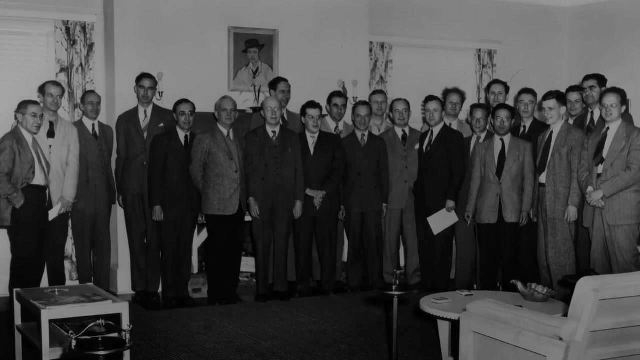 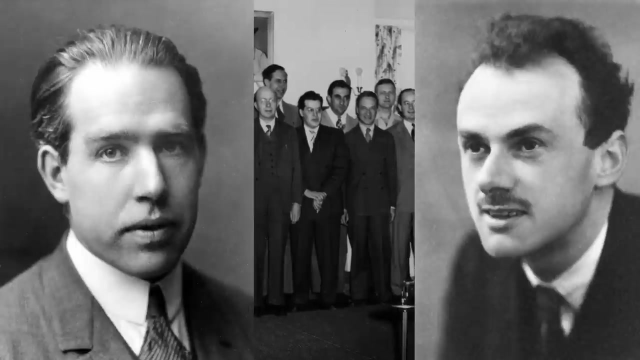 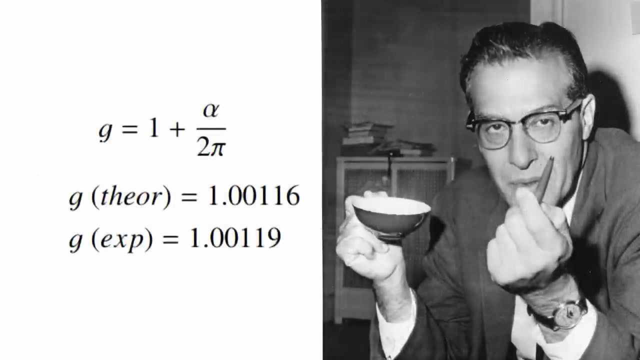 experimentally. At this point you might consider this a mere coincidence but as you will see this coincidence keeps happening and coupled with the fact that he never published any documents explaining his method sets the stage for quite an unbelievable web of deceit. Schwinger's value had a significant impact on the scientific community due to its simplicity and accuracy. Everyone waited in anticipation of Schwinger's theory. None would ever be forthcoming. The following year, 1948, a second conference took place. It was attended by the same participants as the previous one but this time Bohr, Dirac and Fermi attended as well. The conference was focused on Schwinger's presentation. Hopes were high that he would finally present an explanation for how he had calculated the Schwinger factor. When Schwinger finally presented it went on for five hours. 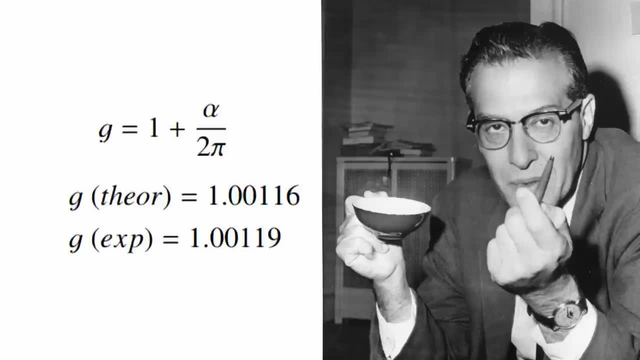 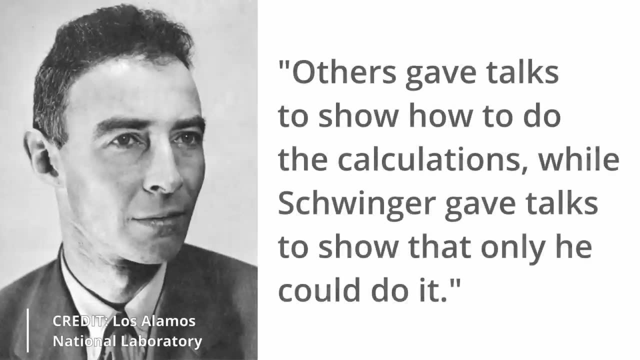 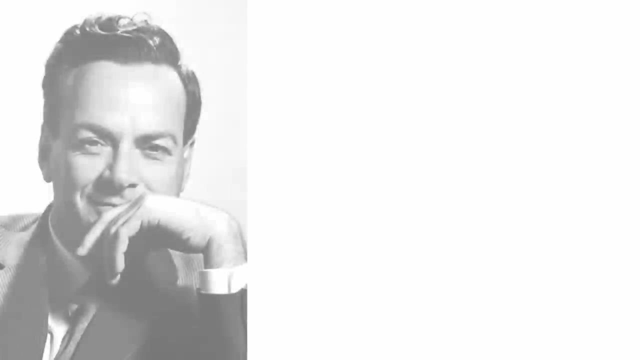 He presented a series of complex and totally incomprehensible equations. Oppenheimer was not impressed saying, others gave talks to show how to do the calculations while Schwinger gave talks to show that only he could do it. The following day Feynman would present his theory and would be the first time to show his famous Feynman diagrams. 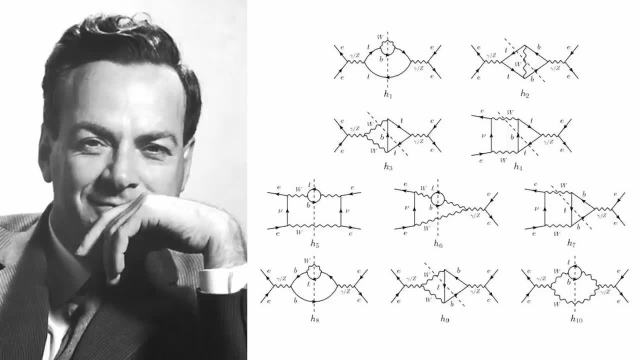 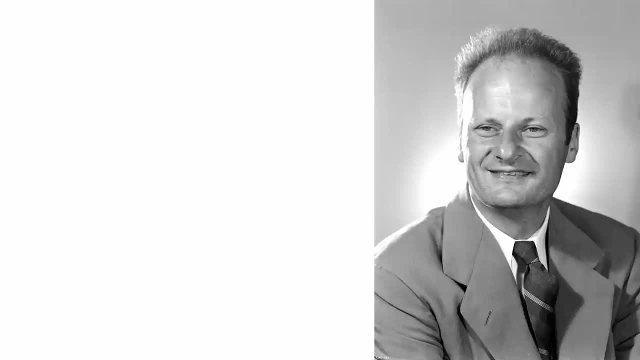 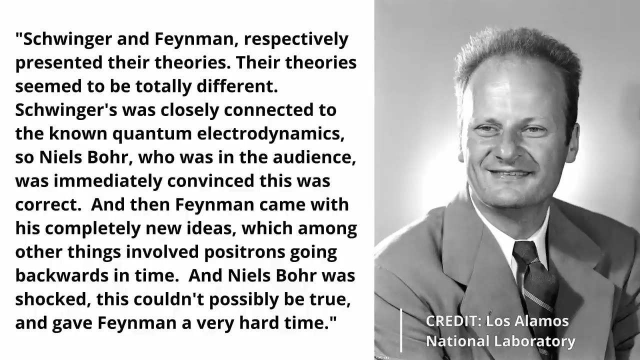 Most attendees did not respond positively to them but Feynman was convinced of the validity of the theory. He was convinced that the theory was true and that the theory was true. Schwinger had the following to say after the conference. Schwinger and Feynman respectively presented their theories. Their theories seemed to be totally different. Schwinger's was closely connected to the known quantum electrodynamics so Niels Bohr, who was in the audience, was immediately convinced this was correct. And then Feynman came along with his completely new ideas 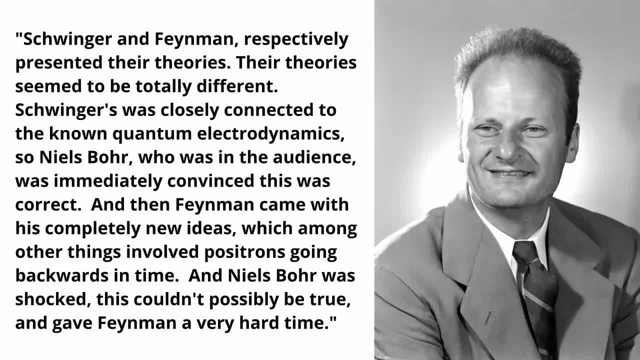 which, among other things, involved positrons going backwards in time. 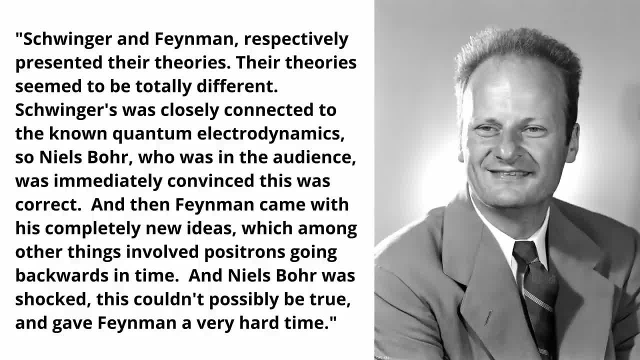 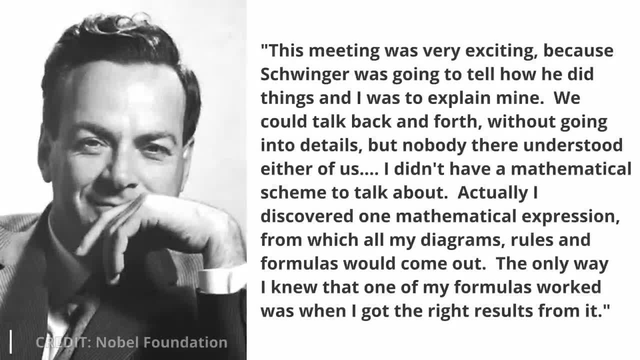 And Niels Bohr was shocked. This couldn't possibly be true and gave Feynman a very hard time. Feynman's recollection is very revealing. This meeting was very exciting because Schwinger was going to tell how he did things and I was to explain mine. We could talk back and forth without going into details but nobody there understood either of us. I didn't have a mathematical scheme to talk about. Actually, I discovered one mathematical expression from which all my data were used. I didn't have a mathematical scheme to talk about. I didn't have a mathematical 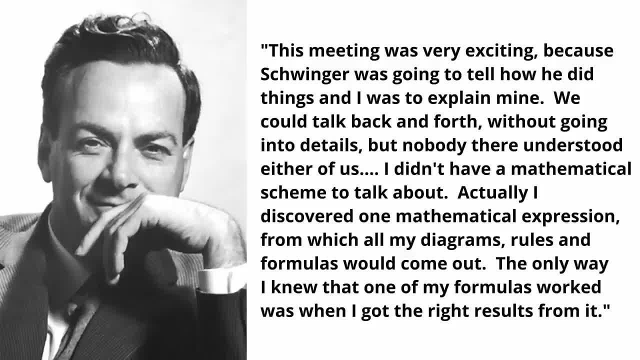 scheme to talk about. All my diagrams, rules and formulas come out. The only way I knew that one of my formulas worked was when I got the right results from it. 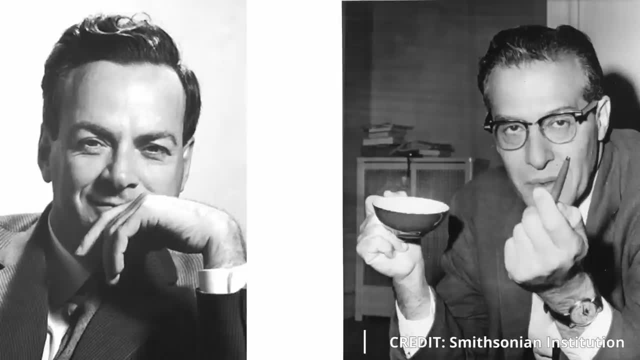 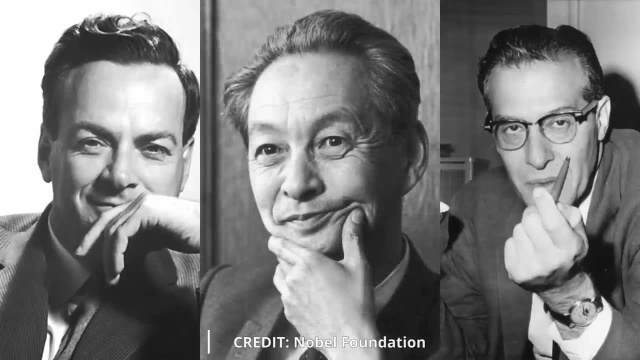 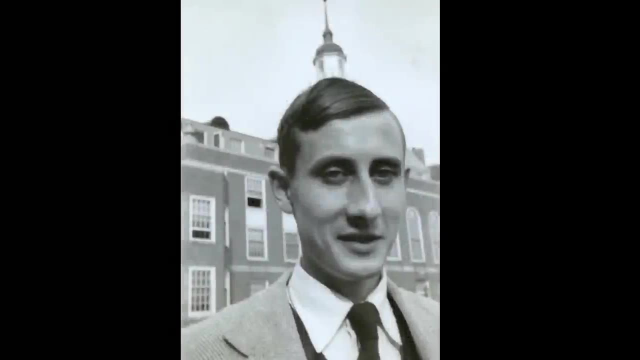 There were now two competing theories for quantum electrodynamics and a third would enter the ring submitted by a Japanese physicist named Tomonaga. The hunt was now on to find a way to unify these theories. The person leading this charge was English physicist Freeman Dyson. Dyson proposed that the Heisenberg scattering matrix could be used to find a way to unify these theories. 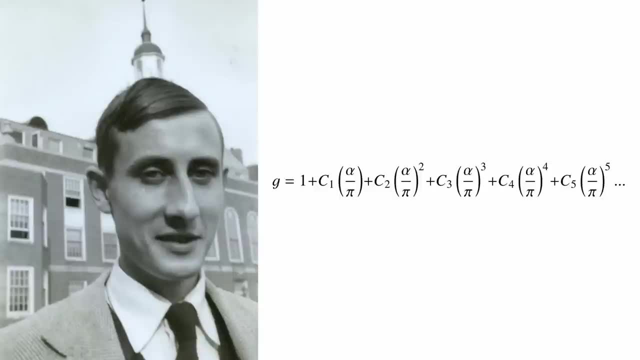 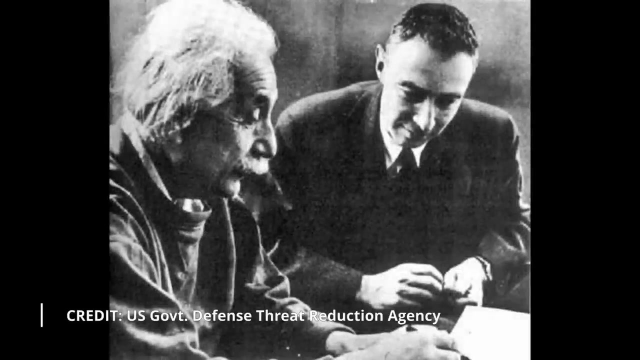 The Heisenberg scattering matrix could be used to calculate the electron's g-factor, transforming it into a series called the Dyson series. The Dyson series was an infinite series of powers of alphas, where the first coefficient was precisely the Schwinger factor, and where each coefficient could be calculated by solving a certain number of Feynman diagrams. By basing his theory on Feynman's diagrams, it provided the solution others had been waiting for. But not all were happy with this approach. Oppenheimer found a way to unify the Heisenberg scattering matrix with a Schwinger factor. Oppenheimer felt that it was entirely the wrong path. He did not believe that Schwinger and Feynman's ideas had much to do with reality. He felt that physics was in need of a radically new idea, and that the quantum electrodynamics of Schwinger and Feynman was just another misguided attempt to patch up old ideas with fancy mathematics. 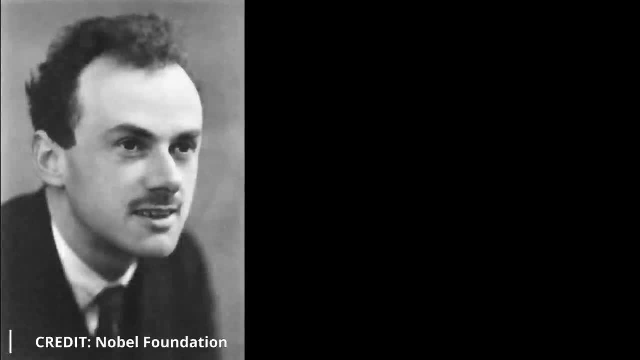 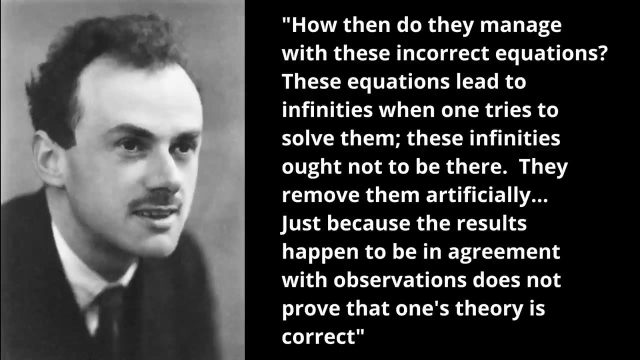 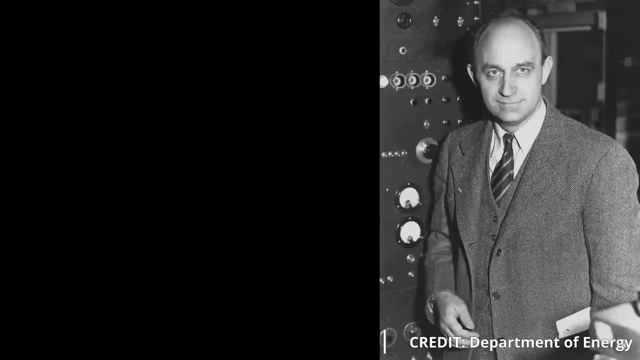 Dirac too felt it was not the correct approach, and stated the following, How then do they manage these incorrect equations? These equations lead to infinity, when one tries to solve them. These infinities ought not to be there. They remove them artificially. Just because the results happen to be in agreement with observations does not prove that one's theory is correct. Fermi was also appalled by the theory. His comment was as follows, 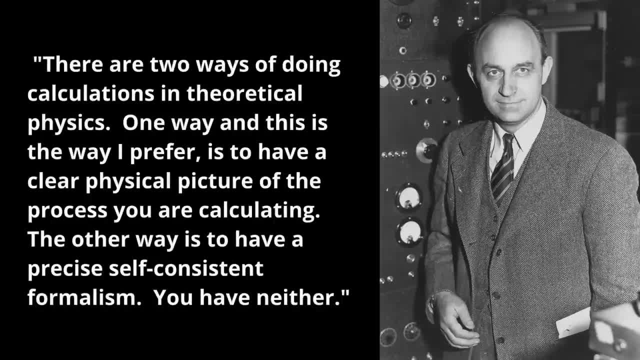 There are two ways of doing calculations in theoretical physics. One way, and this is the way I prefer, is to have a clear physical picture of the process you are calculating. The other way is to have a precise picture of the process you are calculating. The other way is to have a precise self-consistent formalism. You have neither. 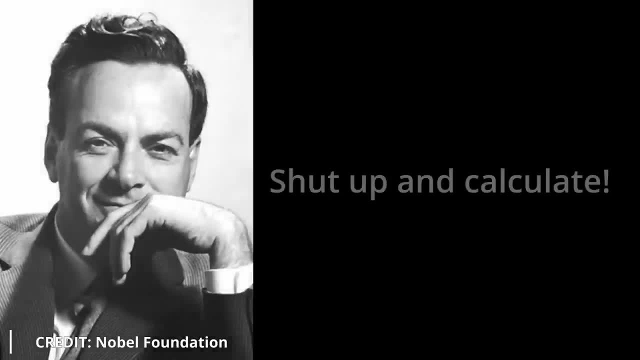 Feynman's response to these critics is well known. Shut up and calculate. The following year, a third conference was held with the same participants. 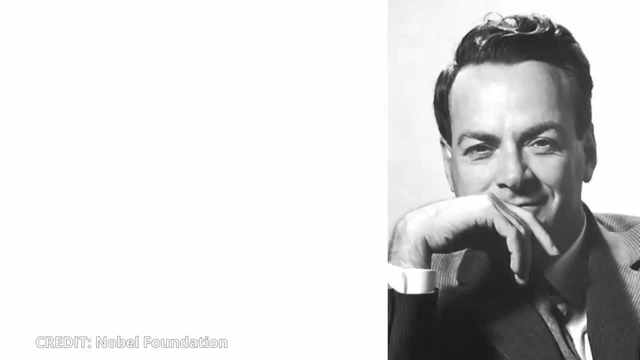 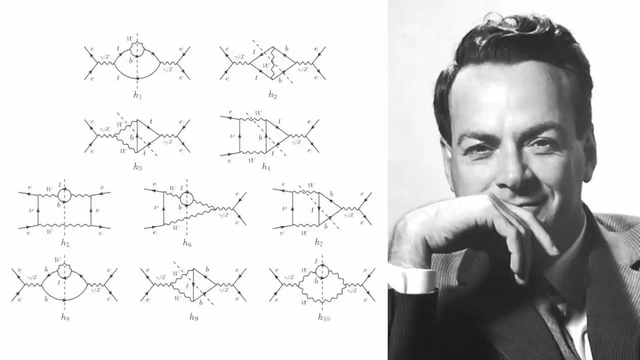 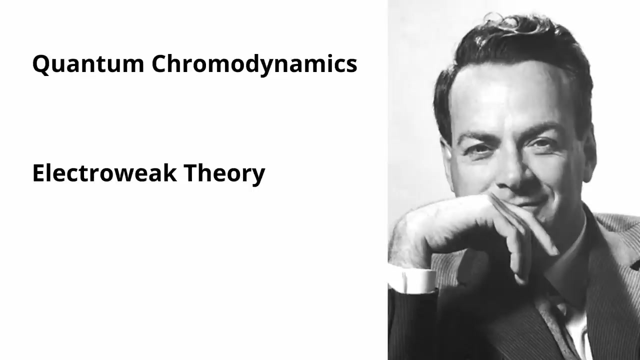 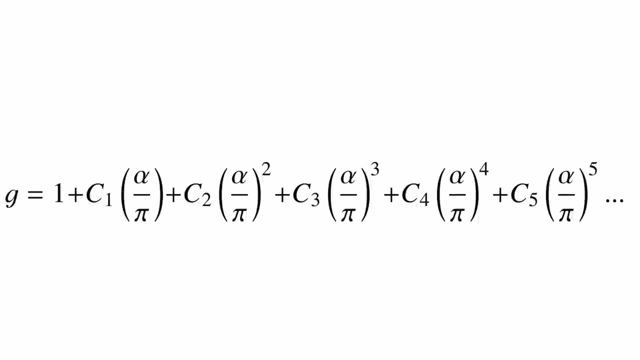 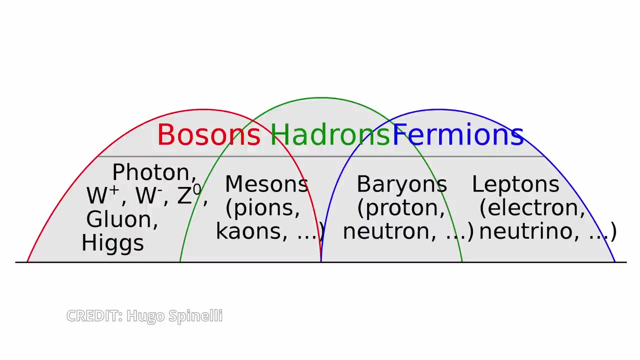 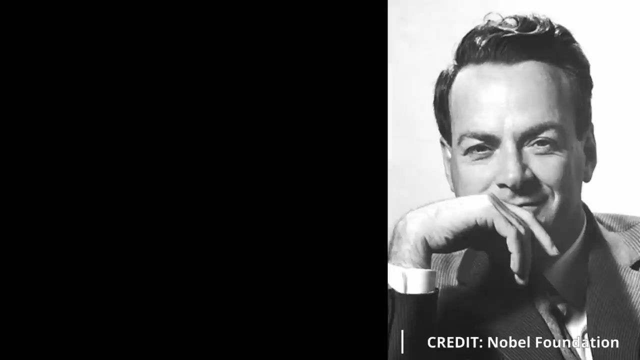 Feynman stole the show with his immense charisma. He presented Dyson's theory as the definitive formalisation of the quantum electrodynamic theory. From that point on, Feynman's diagrams became a popular tool among American physicists, and Feynman took a look at the theory, and he took over as the leader of this new generation of scientists. Further research would result in the formulation of quantum chromodynamics, the electroweak theory, and the standard model of particle physics. But these all rely heavily on the use of Feynman diagrams. These are only valid when the coupling constant has a very low value. If alpha is greater than one, the Dyson series diverges. In the case of fermions, the coupling constant is greater than one. If alpha is greater than one, this means that it is not mathematically legitimate to use Feynman diagrams for the calculations. In 1951, Feynman himself warned of this problem and actually said, 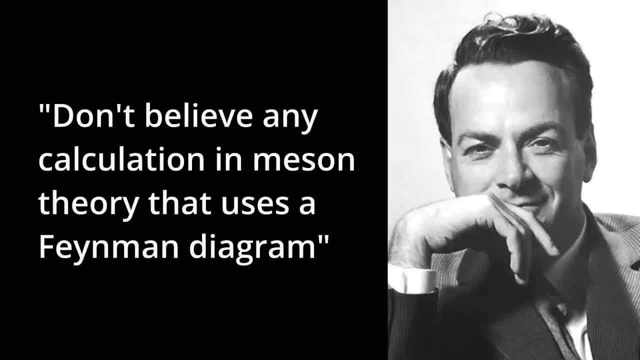 don't believe any calculations in Mison theory that uses a Feynman diagram. 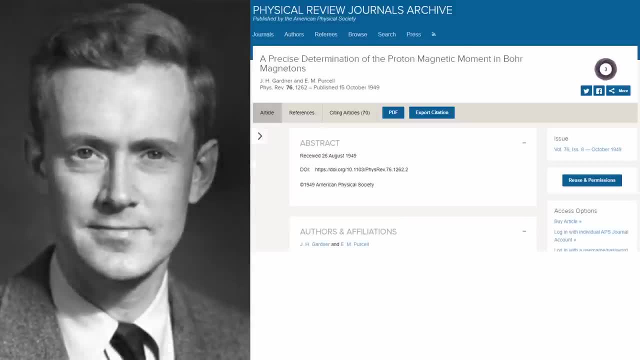 In 1949, Gardner and Purcell obtained a new experimental result for the g-factor 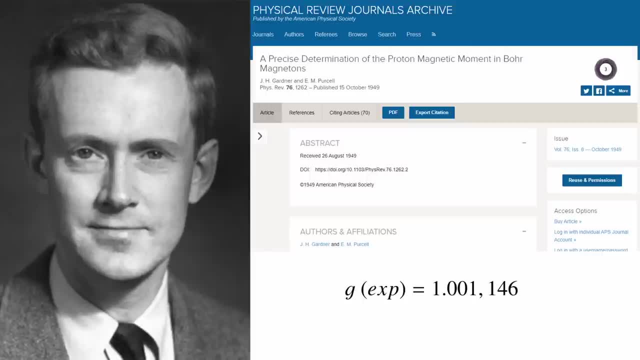 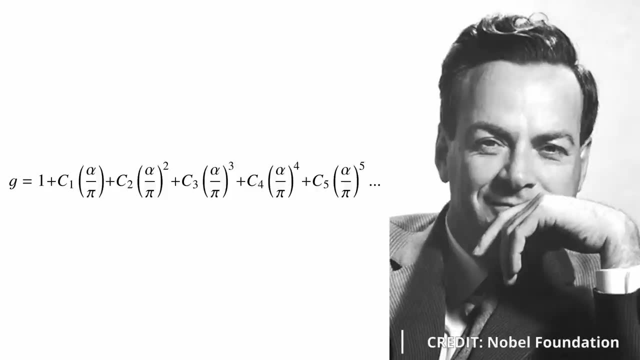 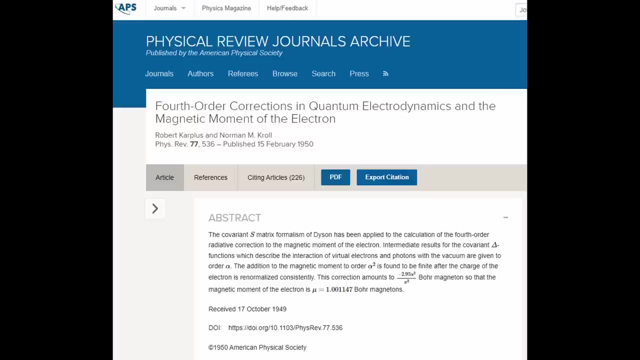 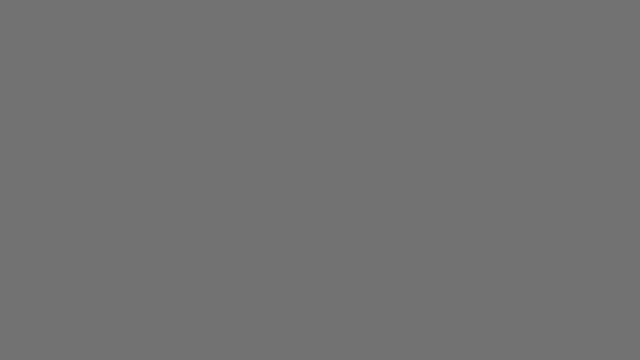 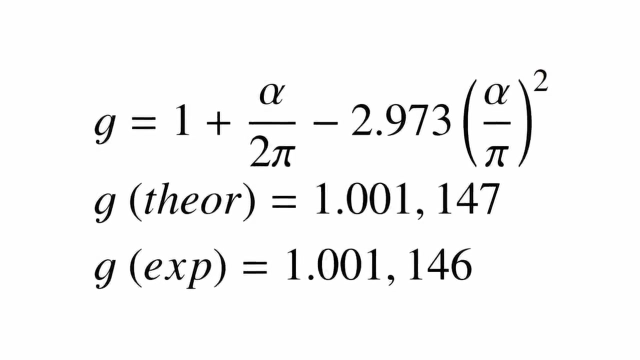 of 1.001146. This now meant that the Schringer factor was no longer considered accurate. This was Feynman's opportunity to push Dyson's theory. A year later, Carplus and Kroll completed the complex calculations and published a value of minus 2.973 for the second coefficient in the Dyson series. For the second time, the new theoretical value was in good agreement with the new experimental value. Quantum electrodynamics had triumphed. Feynman's prestige dramatically 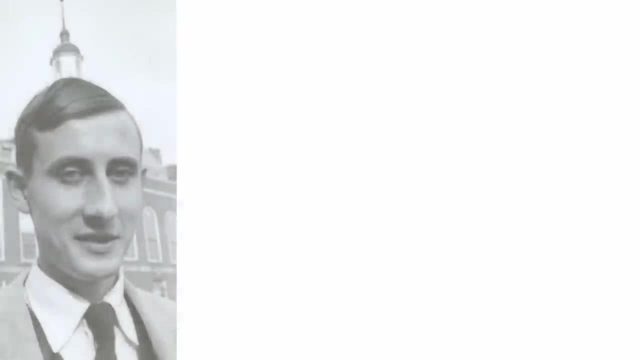 increased. In 1952, Dyson published a paper, titled Divergence of Perturbation Theory in Quantum Electrodynamics. 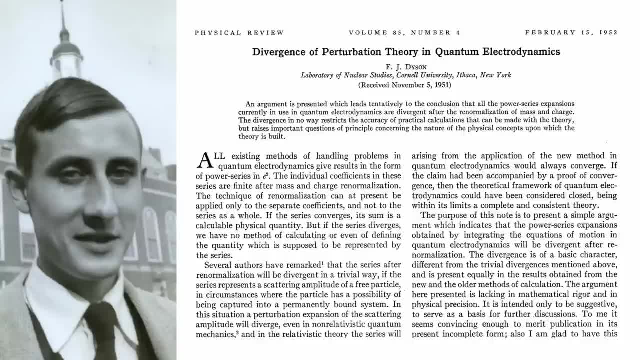 This paper outlined that all the power series expansions currently in use in quantum electrodynamics are divergent after renormalization of mass and charge. 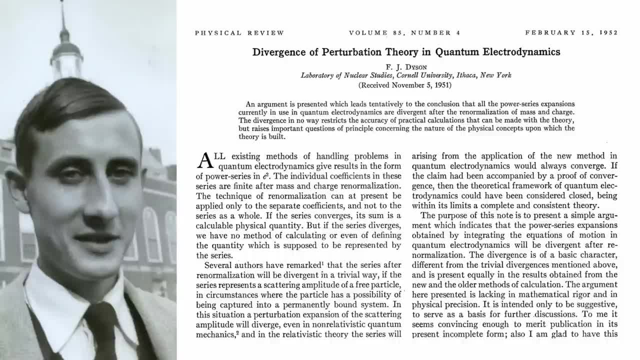 Dyson, the creator of the theory that seemingly fixed the problems in quantum electrodynamics, 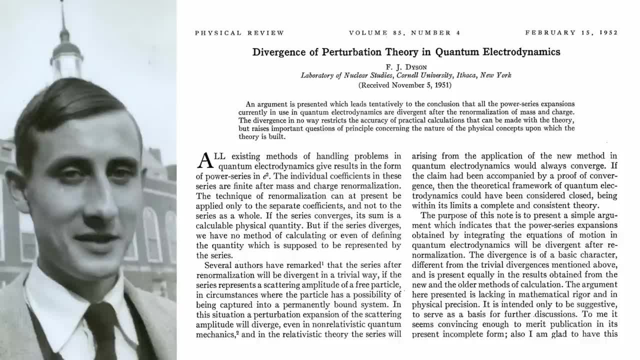 was calling into question the nature of the physical concepts upon which the theory was built. This was a 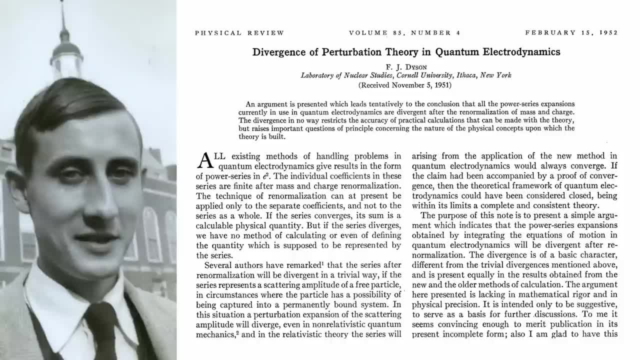 massive blow to Dyson and caused him to move back to England and abandon this line of research in favour of examining other areas in physics. Strangely, no one seemed to pay any attention 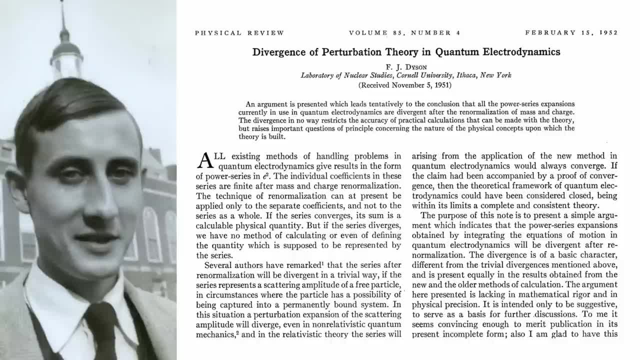 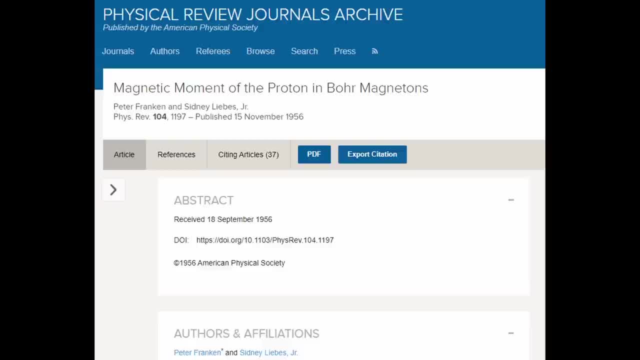 to Dyson's paper, and quantum electrodynamics' credibility was unscathed. In 1956, Franken and Liebes conducted experiments which provided a very different g-factor value, this time 1.001165. 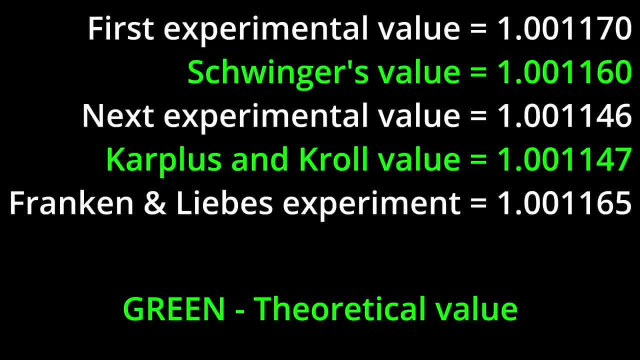 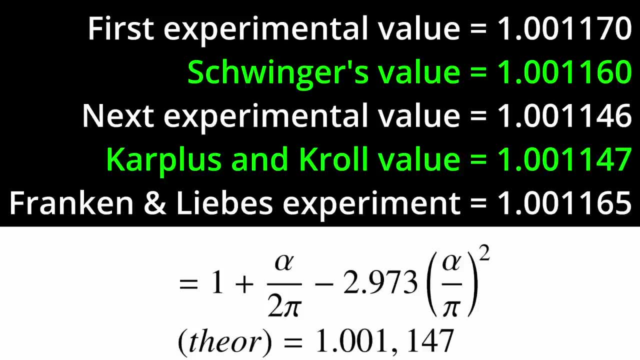 This time, higher than the Schringer factor. This meant that the second coefficient which had been calculated by Kroll and Karpelis actually made the theoretical value worse. Based on the experimental data, this second coefficient should be plus 0.7 instead of minus 2.973. 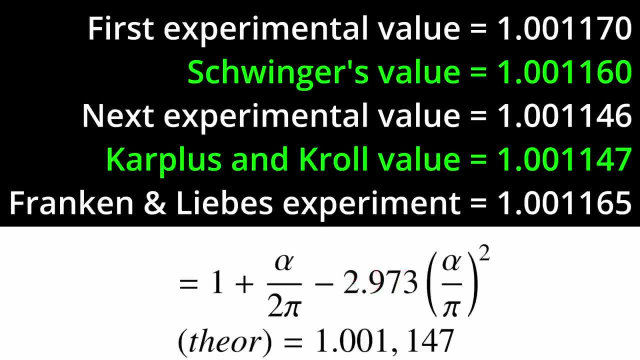 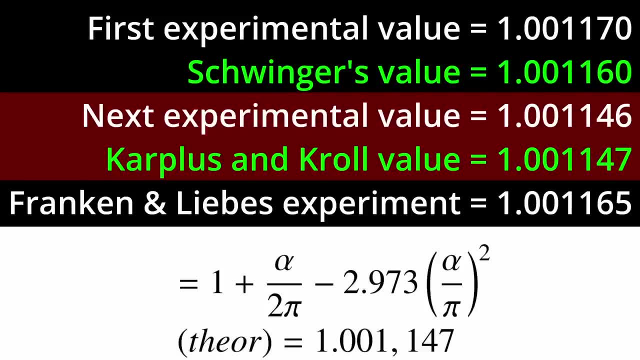 The difference was huge and raised the question of why Kroll and Karpelis' value had provided the exact expected experimental value when the value now turned out to be 0.7. It becomes evident that the quantum electrodynamic calculations had been engineered to match the experimental data. Karpelis and Kroll confessed that they had not independently reached the same result, instead reaching a consensus result and admitted that it was 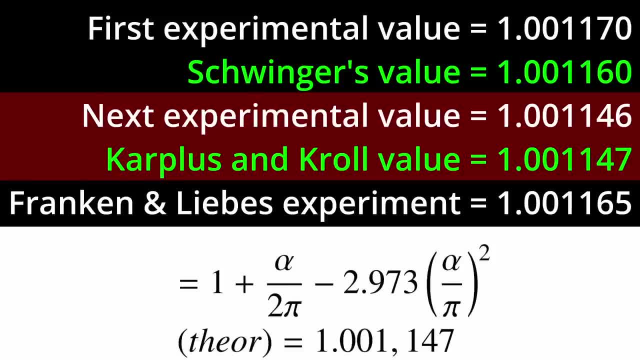 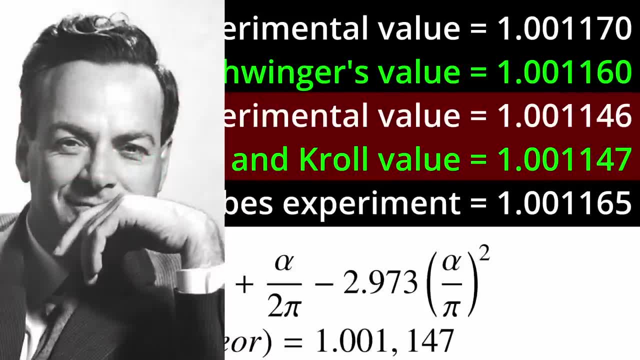 possible that there were errors in the calculations. Feynman would later claim that this was merely a mistake in arithmetic. And once the mistake was found, all was once more in agreement. 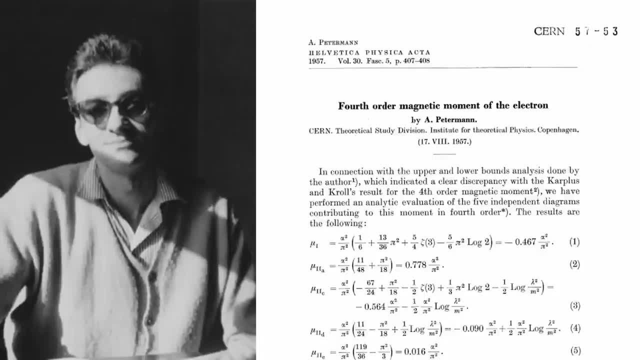 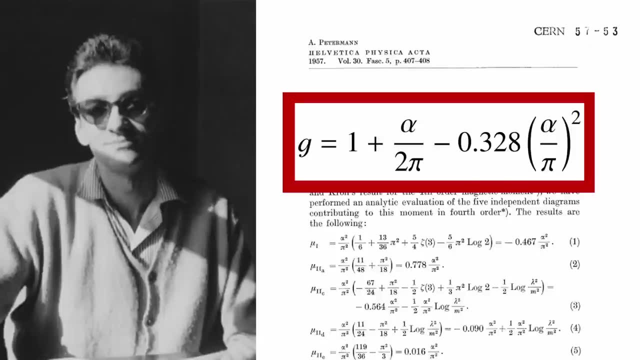 Seven years after Kroll and Karpelis first published their paper, Peterman detected another error in their calculation. When he then corrected this mistake, he obtained a result of minus 0.328, which was almost 10 times smaller than the 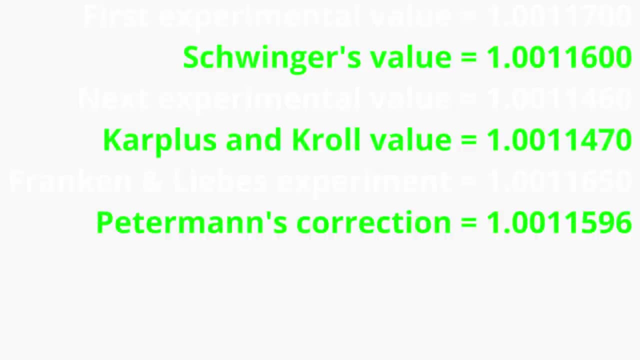 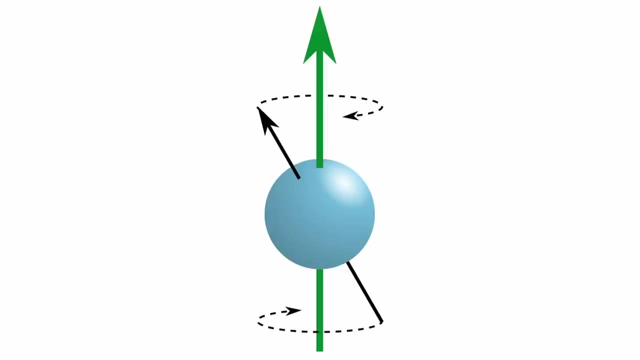 original value. In 1953, a new type of experiment was proposed to calculate the magnetic moment of the electron directly from the precession of the free electron spin. In 1961, based on this method, Schupp, Pidd, 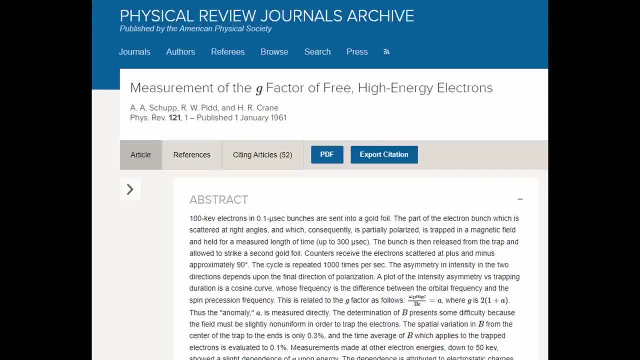 and Crane carried out the experiment and obtained a new value of 1.0011609. 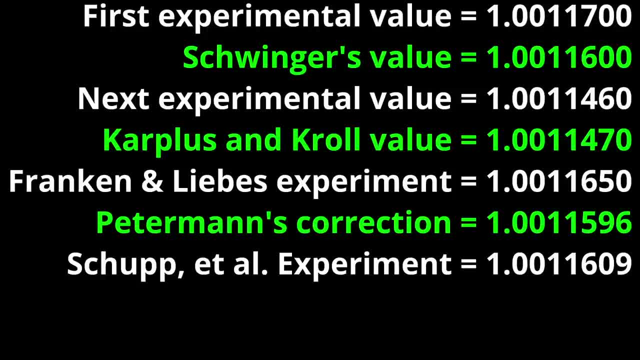 This method should have provided a much more precise measurement, but the authors were very cautious and used a large margin of error. 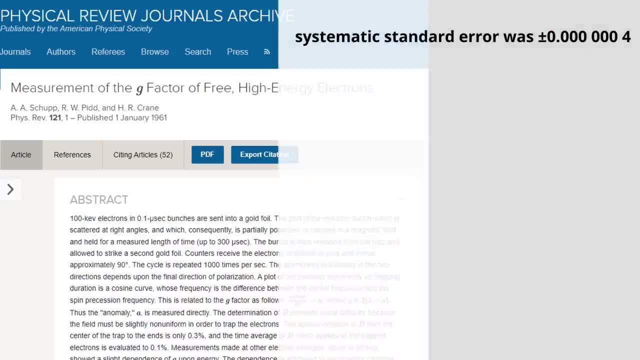 The estimated systematic standard error was 0.0000004. If they had used this error, it would have meant Peterman's theoretical value was outside the standard value. 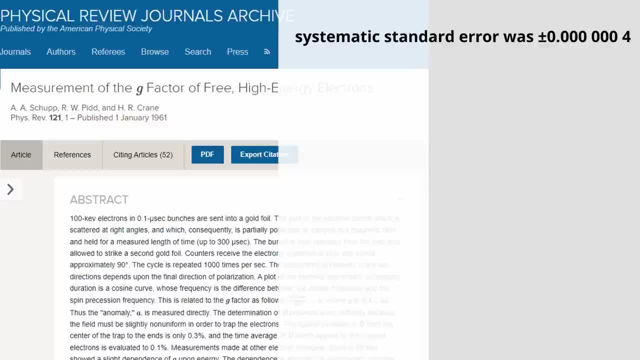 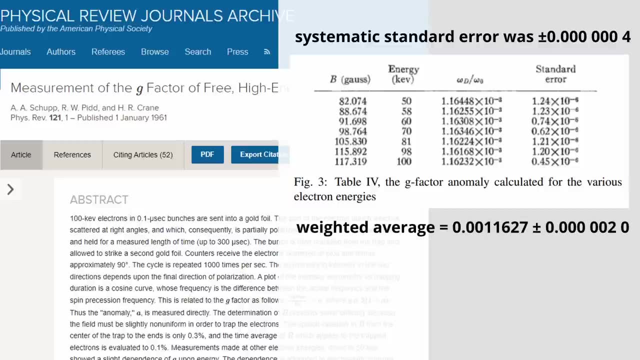 They conducted a series of runs for different electron energies. The weighted average of this is 0.0011627 plus or minus 0.000020. This falls outside of Peterman's theoretical value. 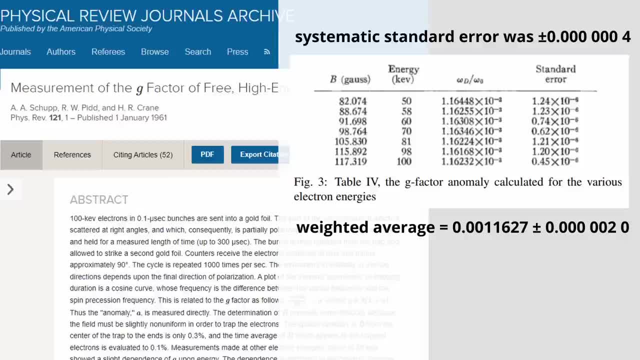 So how did they come up with a single value? They felt they needed to recognise the trend of error. They felt they needed to recognise the trend of error. 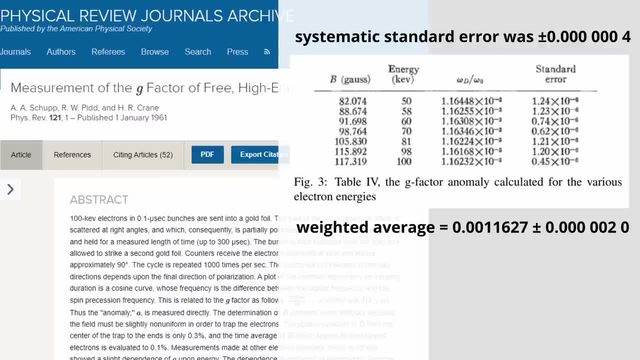 They felt they needed to recognise the trend of error. So the way they were able to obtain a value that still aligned with Peterman's one is by taking this single value, adding the error from that to the averaged error to obtain a final value 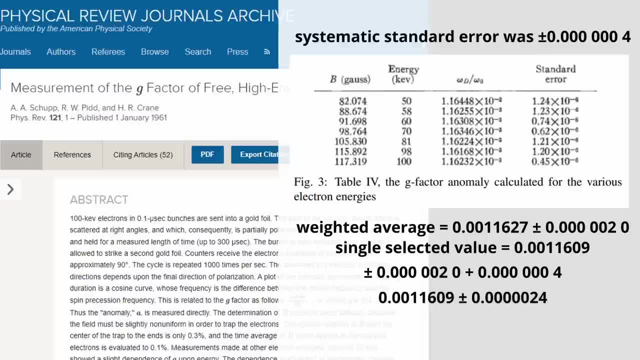 of 0.0011609 plus or minus 0.0000024. 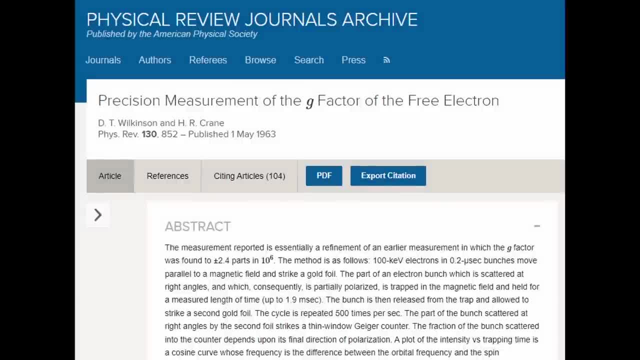 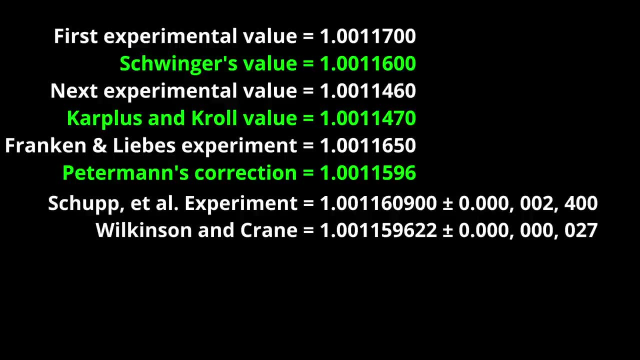 Two years later, in 1963, Wilkinson and Crane published an improved version of the experiment, this time the value was 1.001159622 plus or minus 0.00000027, nearly the same as Peterman's theoretical value. 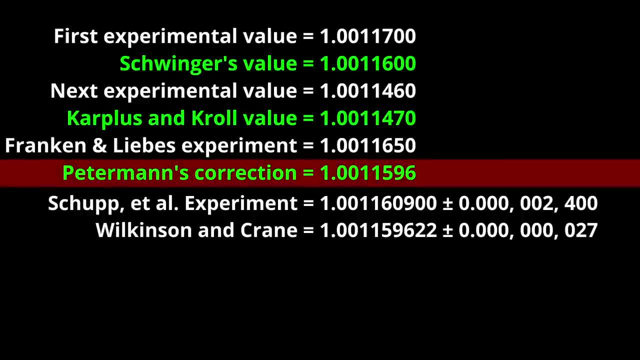 This experiment was conducted at the same university with the same team. This makes it very strange that all the measurements from the previous experiment were outside of the range of the new experimental value. 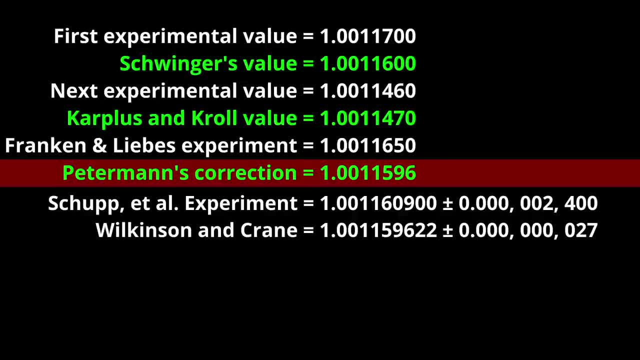 It also fits perfectly with the theoretical value. The most disturbing aspect is that 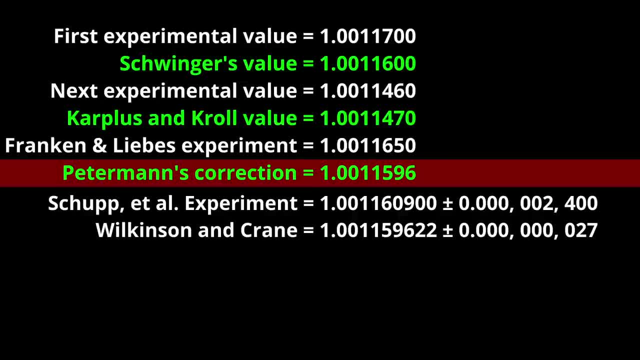 the value is not correct, as was demonstrated in later experiments. 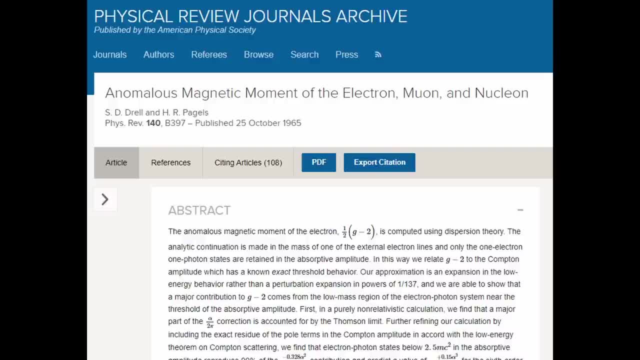 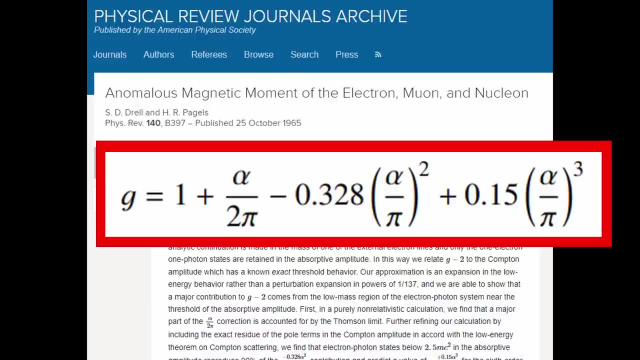 In 1965, Drell and Pagels published the first calculation of the third coefficient of the Dyson series. This required solving 72 Feynman diagrams. The result was 0.15 and resulted 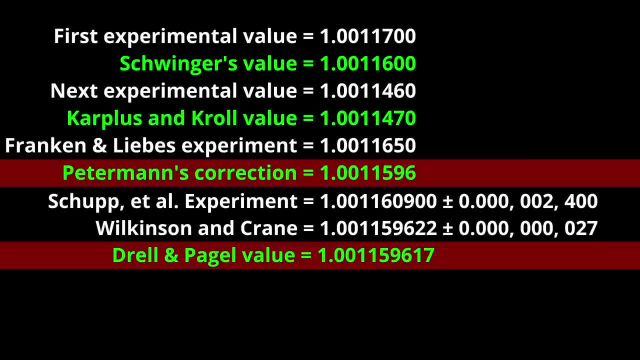 in a slight change to the value of the electron g-factor. 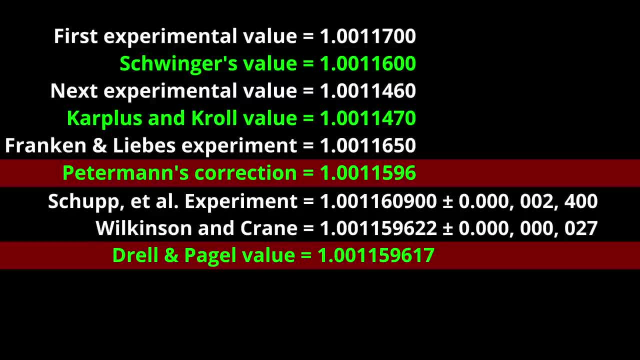 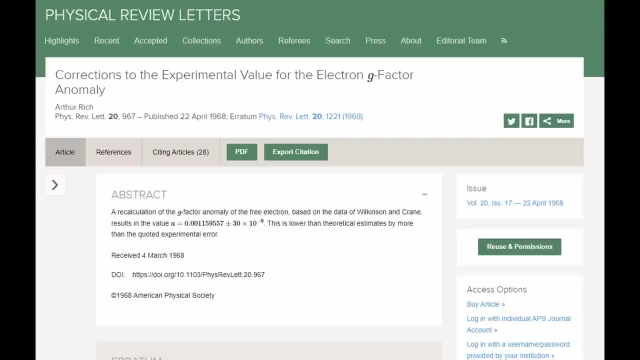 Based on this, all doubts about quantum electrodynamics were cleared. Feynman, Schwinger and Tominaga were awarded the Nobel Prize in Physics. In 1968, Rich re-evaluated the Wilkinson experiment 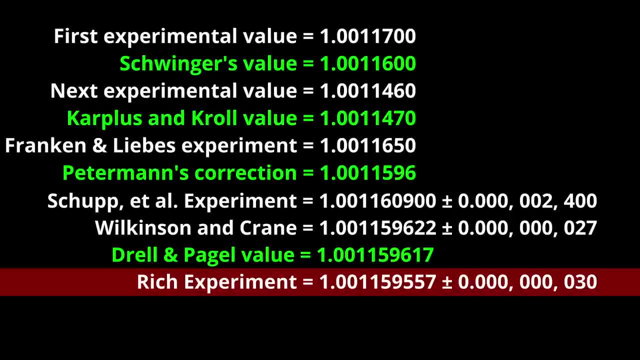 and obtained a different result. Other researchers would find further errors in the experiment. 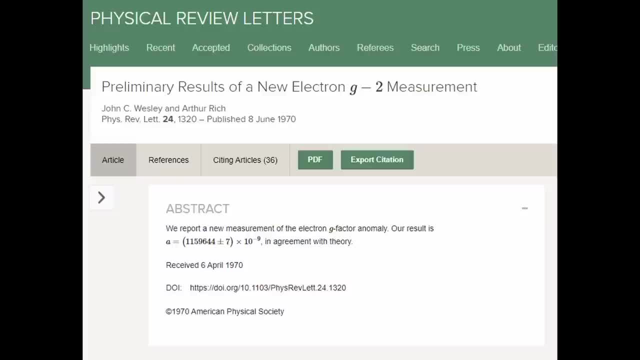 Two years later, Rich and Wesley repeated the experiment, fixing the detected ambiguities and obtained a result higher than the previous one. 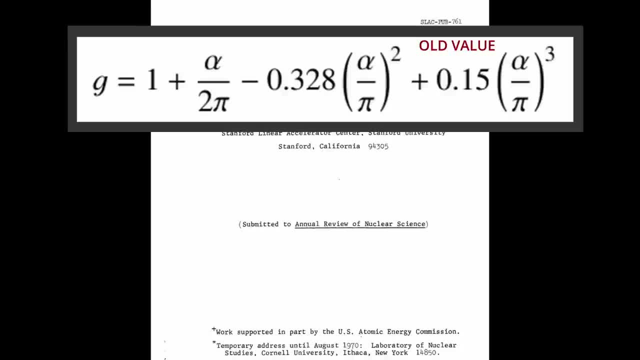 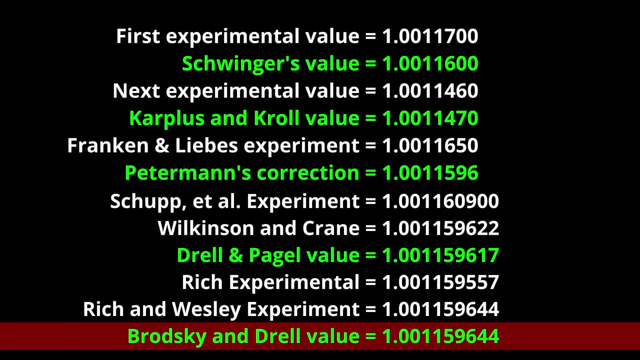 That same year, Brodsky and Drell published the first calculation of the third coefficient of the Dyson series. Brodsky and Drell recalculated the third coefficient and obtained a different value, three times higher than the previous one. Conveniently, the new coefficient and the new experimental value were once more in agreement. 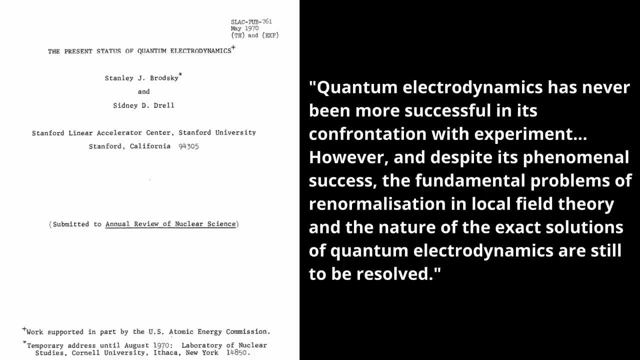 Brodsky and Drell summarise the situation as follows. Quantum electrodynamics has never been more successful in its confrontation with experiment. However, and despite its phenomenal success, the fundamental problem of renormalisation 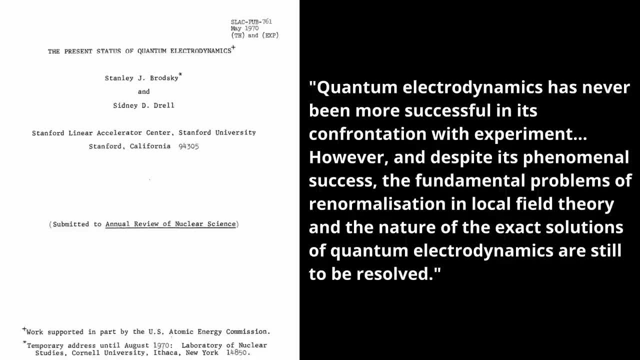 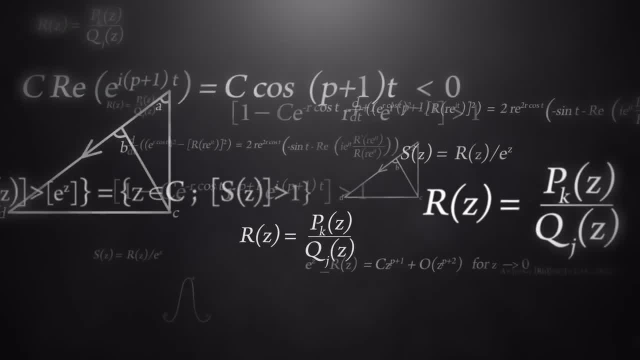 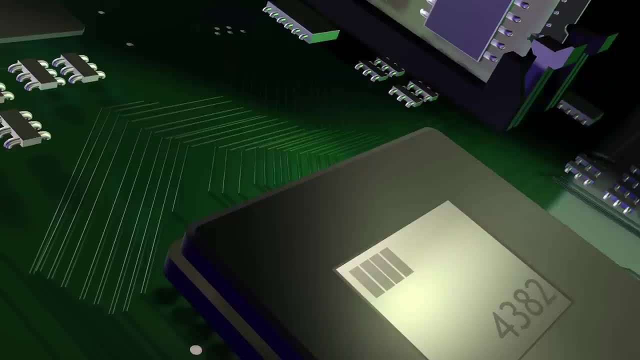 in local field theory and the nature of the exact solutions of quantum electrodynamics are still to be resolved. From this point onwards, all the mathematical calculations required to obtain the coefficients of the Dyson series would be performed by computer. No source code for these calculations has ever been published, making it impossible to reproduce 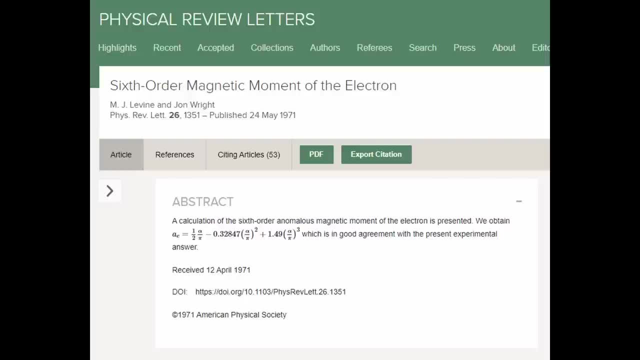 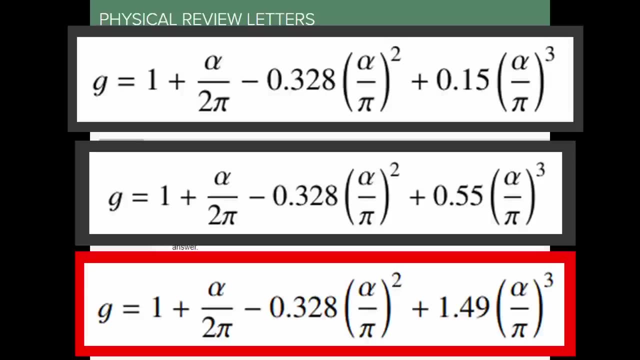 any calculations independently. In 1971, Levine and Wright recalculated the third coefficient, and once more, it was three times higher than the previous one. 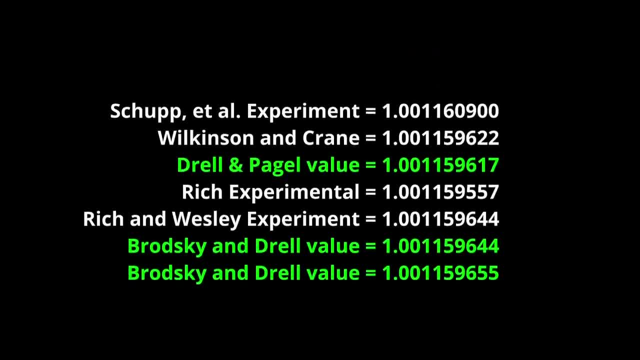 The same year, Wesley and Rich published their final results for the experiment as the previous results had apparently only been preliminary. Their final results were slightly higher than 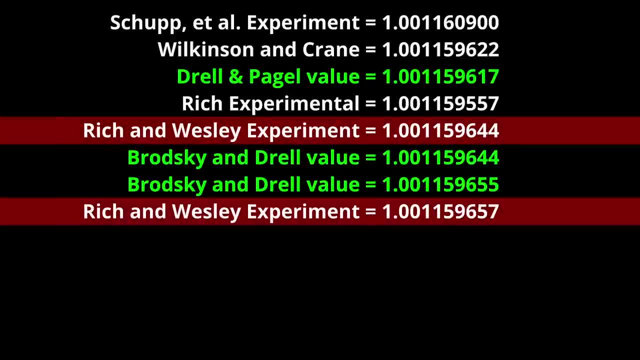 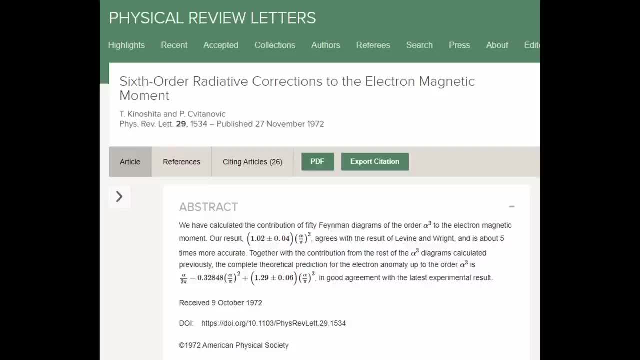 the previous one. By another striking coincidence, this new coefficient and the new results once more seemed to match up. A few months later, Kinoshita and Kvitanovic published a new calculation 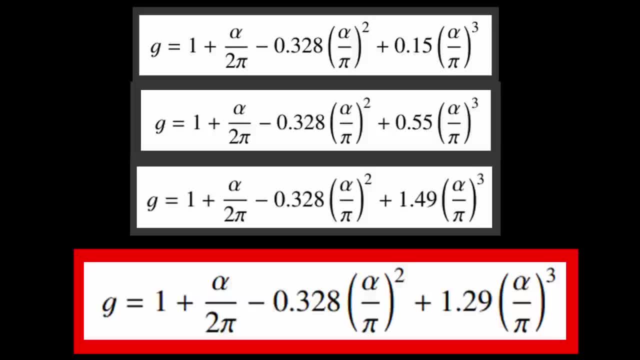 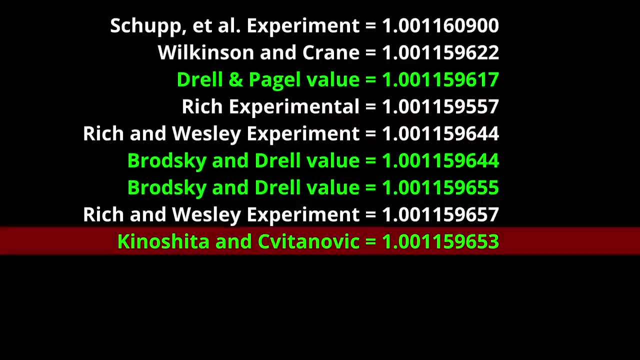 for the third coefficient. They claimed it was five times more accurate than Levine and Wright's previous one. This time, it was slightly lower, and made the agreement with the experimental 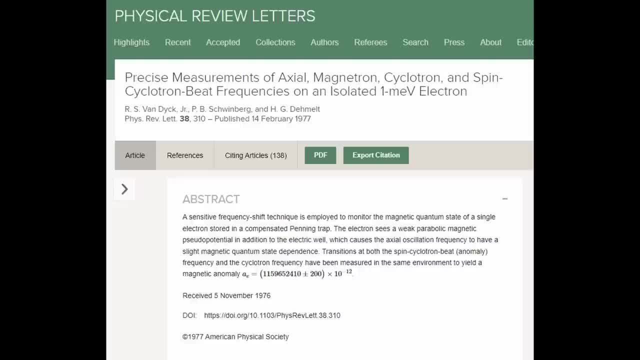 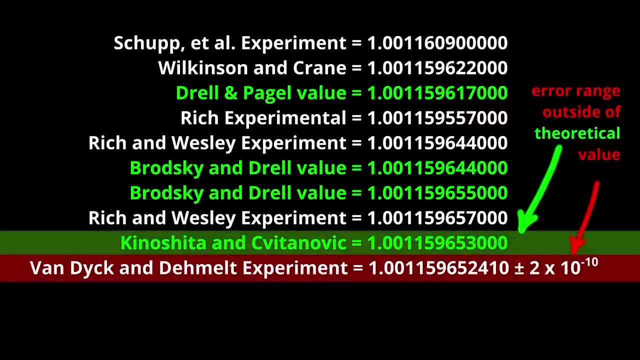 value slightly worse. In 1977, Von Dyck and DeMelt used a new technique to obtain a new experimental value. Once more, the experimental results did not match the theory. In order 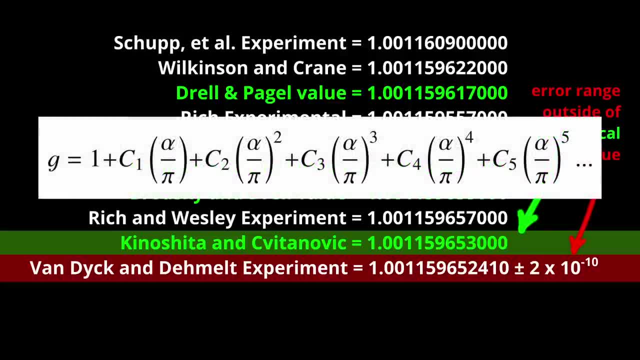 to resolve this, the theoretical physicists felt they needed to calculate the fourth coefficient. 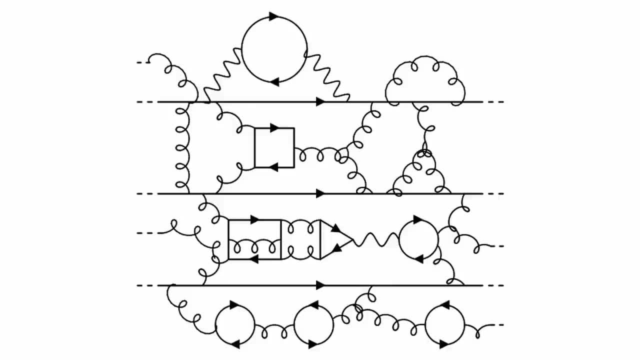 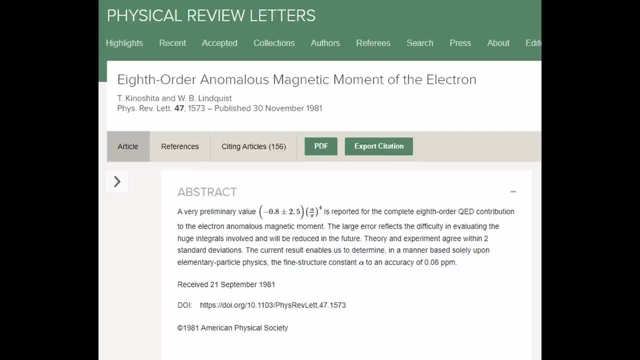 This involved solving 891 Feynman diagrams. Four years later, Kinoshita and Lindquist published the first calculations of the fourth coefficient, with a value of minus 0.8. 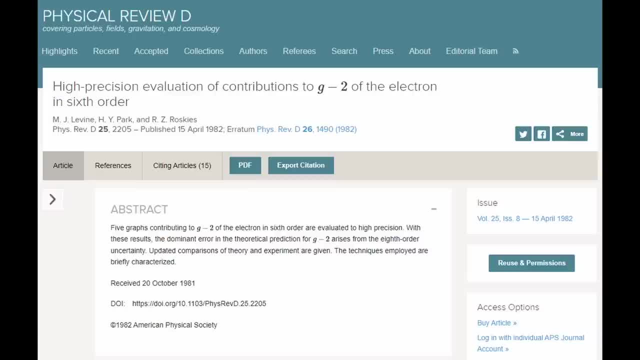 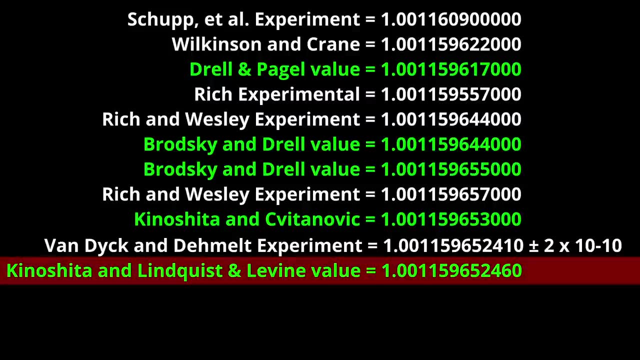 But then, in 1982, Levine published a new calculation of the third coefficient, and again, it was lower than the previous one. This once more brought the theoretical value 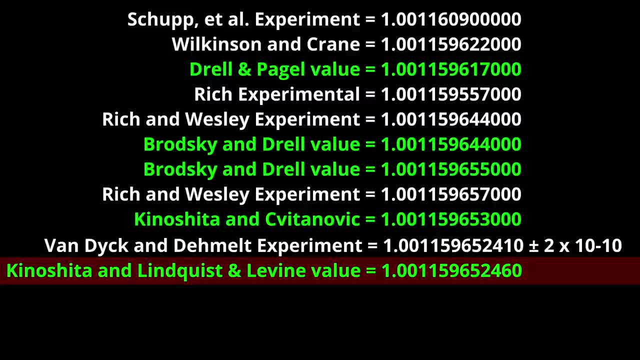 in line with the experimental one. Von Dyck and DeMelt published 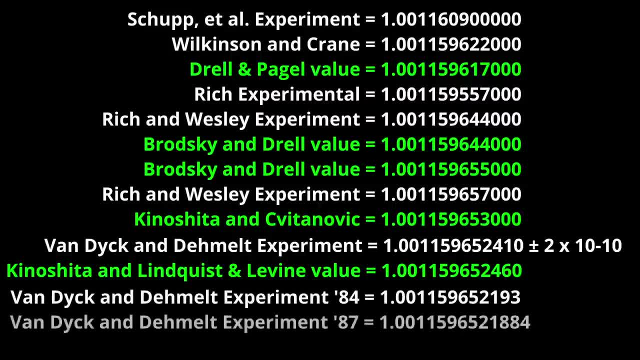 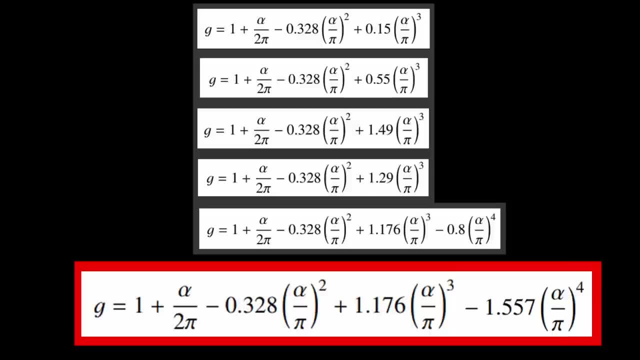 two more results in 1984, and then again in 1987, and once more brought the experimental value out of line with the theoretical one. In 1995, Kinoshita's team published a new value 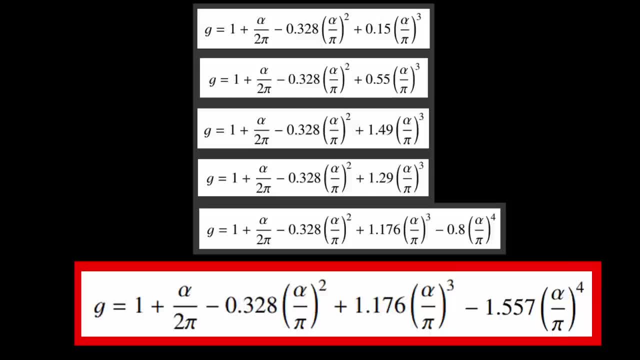 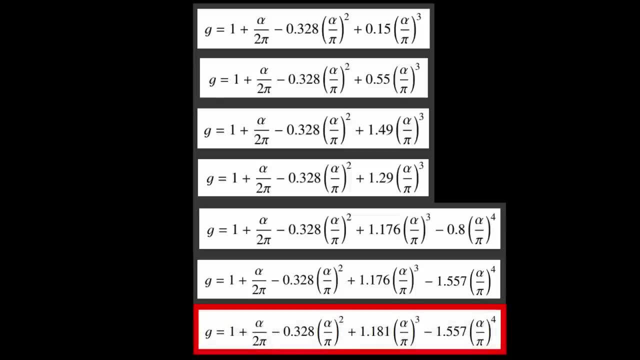 for the fourth coefficient, almost double their previous value at minus 1.557. The following year, Laporte and Remedy would publish a new value for the third coefficient, at plus 1.181. 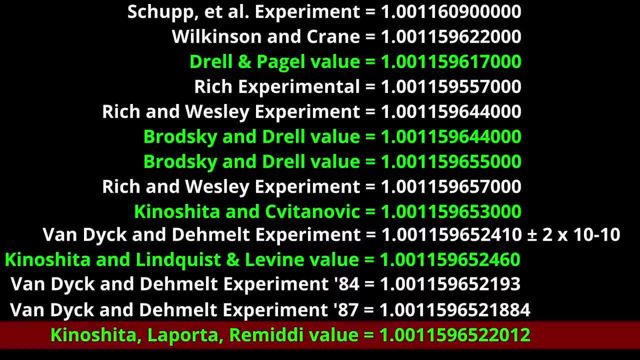 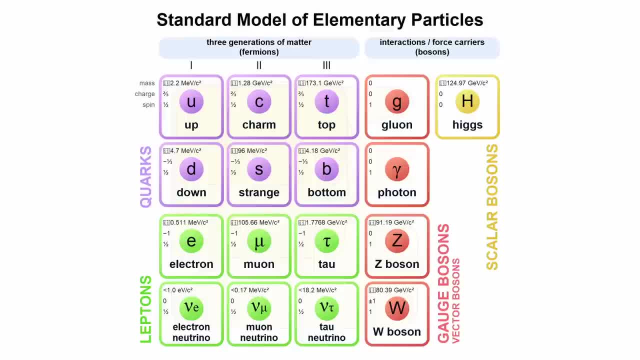 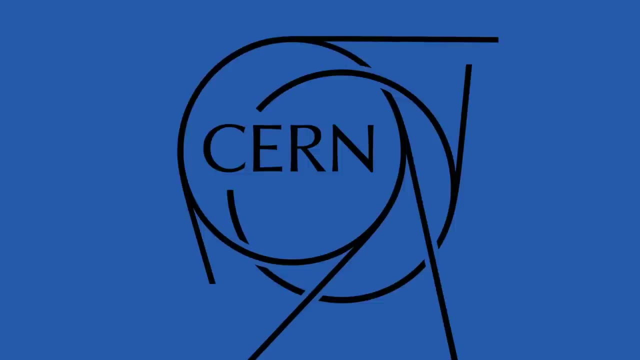 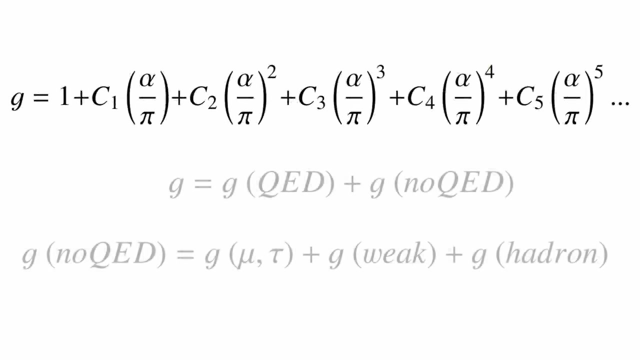 These would once more bring experimental results in line with the theoretical. The muon's g-factor. A muon is almost identical to an electron, except that it seems to have a much greater mass. Quantum electrodynamics was used to calculate the anomalous magnetic moment of the muon. A muon is very unstable, making high-resolution measurements very difficult. CERN made the first measurements and unfortunately the theoretical value did not match the experimental one. In order to solve this problem they decided to add in adjustment factors. These factors would be taken from the standard model of particle physics. The first coefficient would be derived from the interaction of the electron with a lepton, the second from the electroweak interaction and the third from the interaction of the electron with hadrons. These factors unsurprisingly did bring the new theoretical value much closer in line with the experiment. 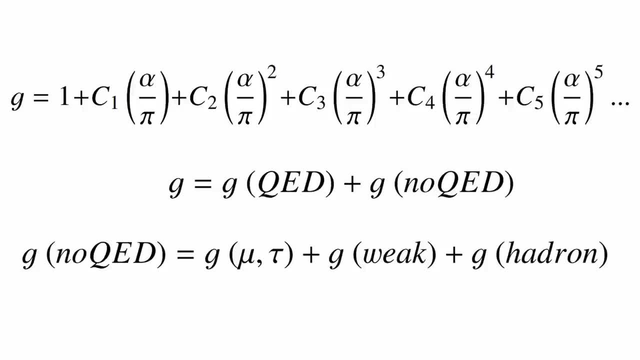 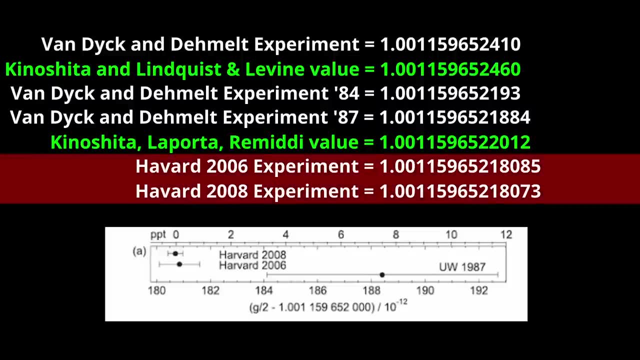 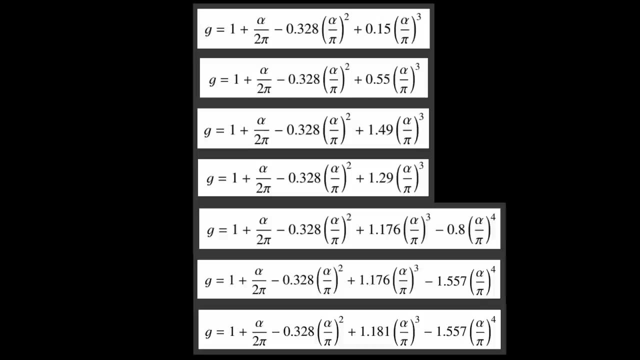 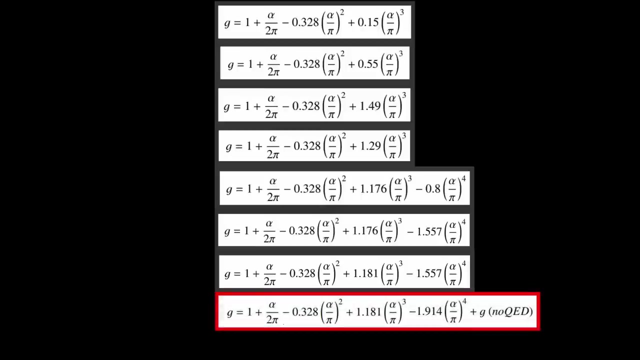 This change unfortunately made the theoretical electron g-value worse and this created yet another discrepancy. In 2006 Harvard improved the electron measurements even further. In 2007, Kinoshita's team detected an error in their previous calculations of the fourth coefficient. They had found an inconsistency in the old treatment of infrared subtraction terms in two diagrams. When they corrected for this, the new value came out as minus 1.914. With these changes, the new theoretical value was once more in good agreement with the new experimental value. 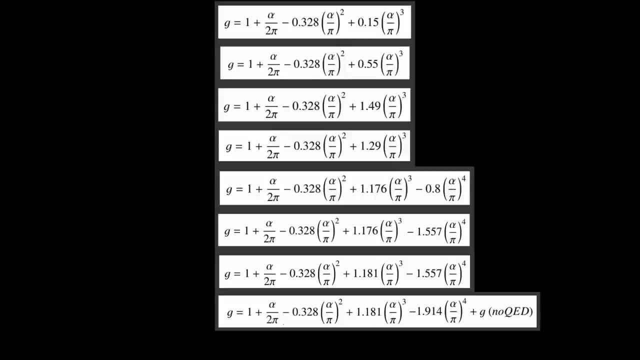 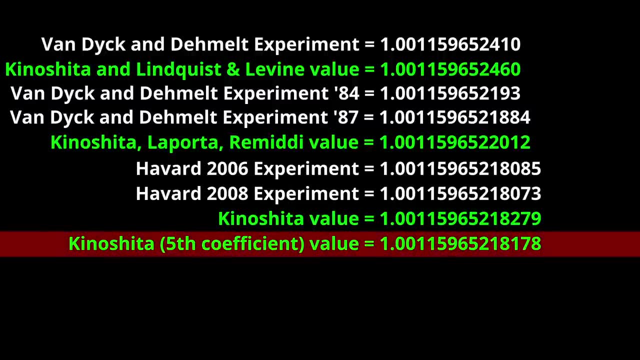 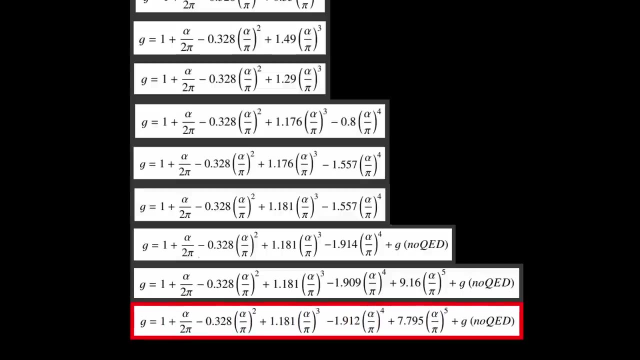 In 2012, Kinoshita's team published the first fifth coefficient. This involved calculations based on 12,672 Feynman diagrams. They also published a slightly improved value for the fourth coefficient. Three years later, they would publish an improved value for both. 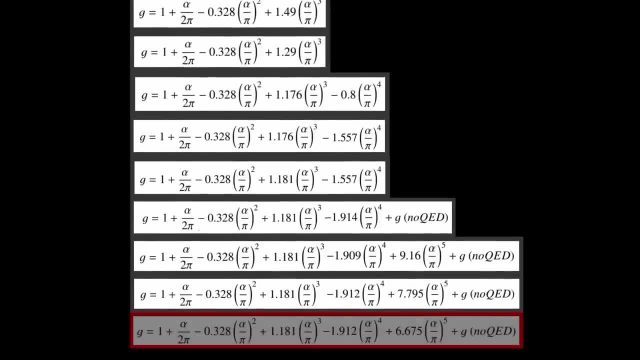 Then, in 2018, they once more detected an error in their previous calculations of the fifth coefficient. 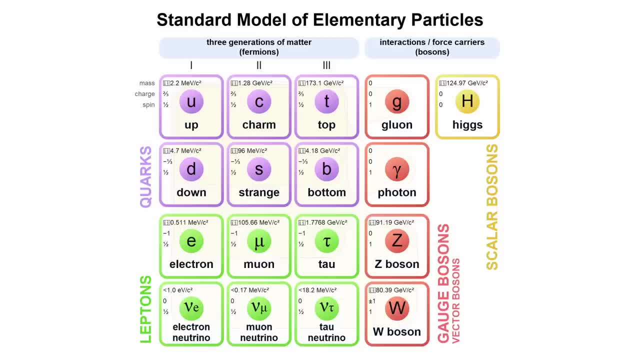 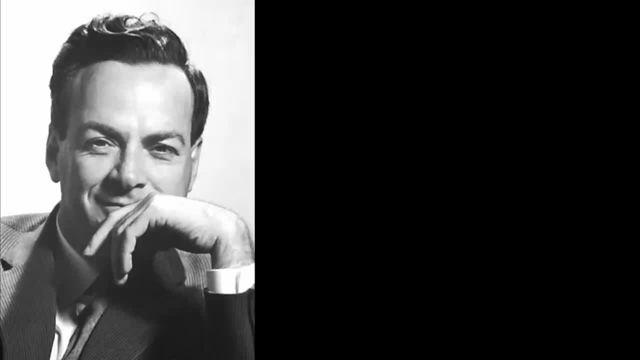 All the while these corrections were ongoing, the Muon g-factor experimental results refused to come into line with theoretical predictions. These persist even today. 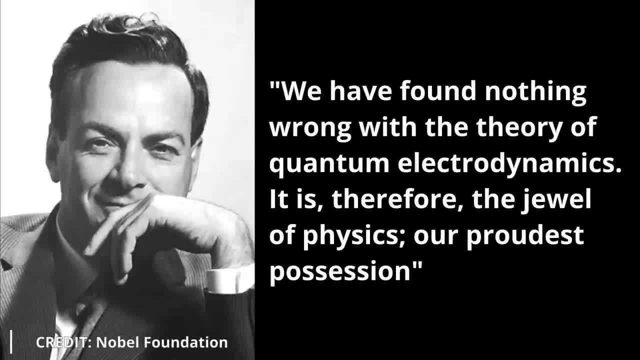 According to Feynman, we have found nothing wrong with the theory of quantum electrodynamics. It is therefore the jewel of physics, our proudest possession. But maybe the sentiment 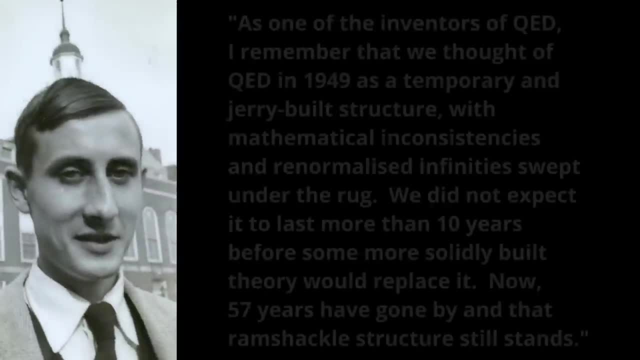 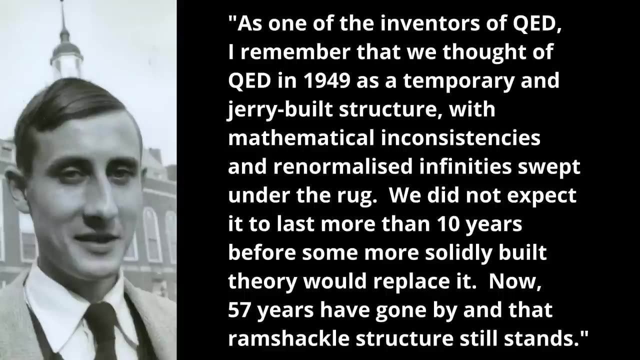 is better portrayed by Dyson, who wrote in 2006, as one of the inventors of quantum electrodynamics, I remember that we thought of quantum electrodynamics in 1949 as a temporary 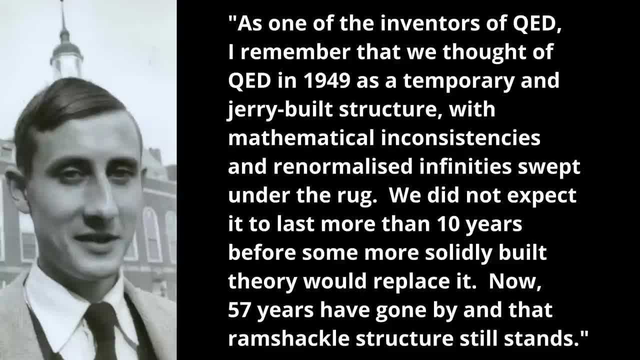 and jerry-built structure, with mathematical inconsistencies and renormalised infinities swept under the rug. We did not expect it to last more than ten years before some more solidly built theory would replace it. Now fifty-seven years have gone by and that ramshackle structure still stands. We are now in the middle of a new era of quantum electrodynamics. We